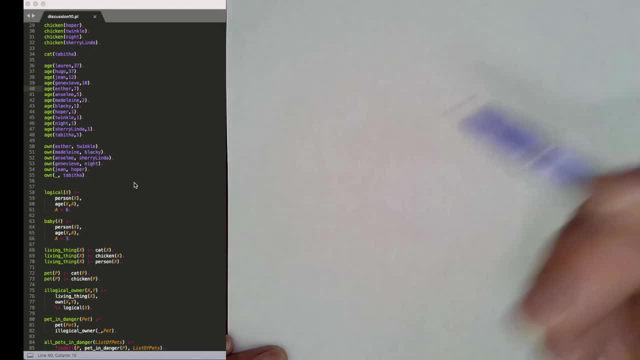 but before we get into Prologue as such, let me start by saying giving you a little bit of background in terms of what the field of resolution and solving problems in logic in general, Just so you know, you've probably heard of propositional logic, you know. 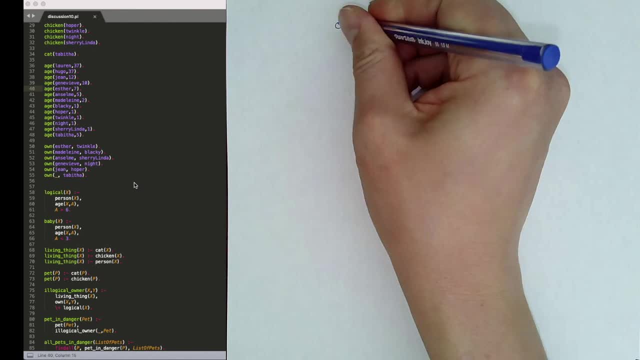 like propositions like A or B, things like that. But we can you know, solving this problem is called a satisfiability problem. It's quite simple. It consists in figuring out what are the truth values of A and B that are such that this whole proposition is true right? 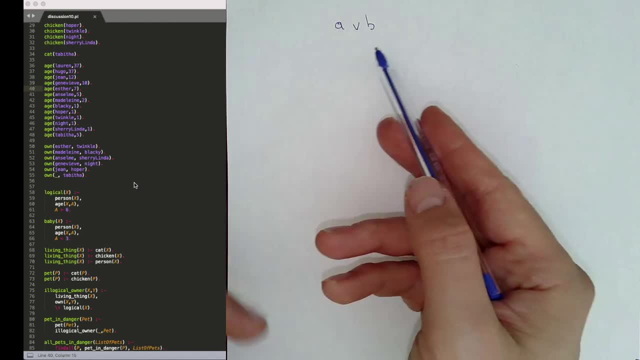 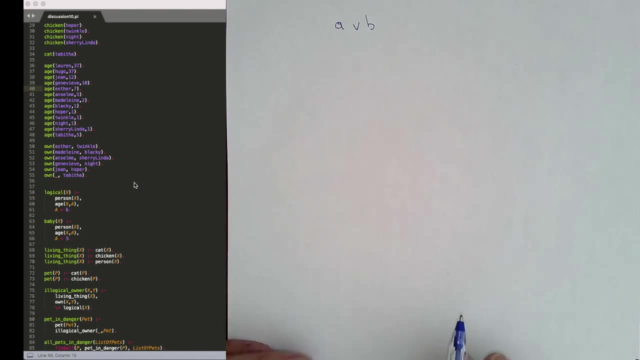 So here there are multiple. You can have: A is true or B is true or both are true. In these three cases it works. Sorry, in these three cases it works and it's satisfiable. OK, in this field in general. you have to be aware that it's important to understand that problems are very, very hard to solve. 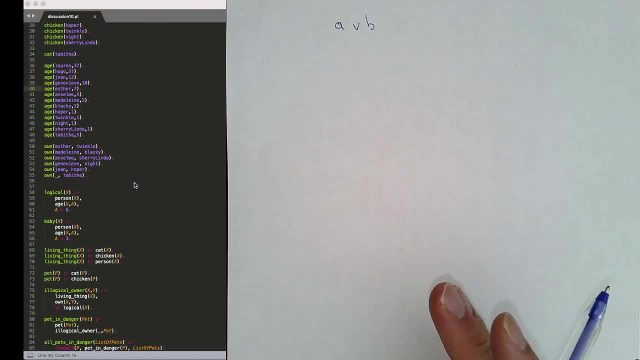 And in general they are just intractable problems. So if we take- what I mean is that if we take any kind of logical proposition of any arbitrary size or style, it will be. it will take an exponential time to solve Why. Because so if we take a proposition only in the form of what we call clauses, 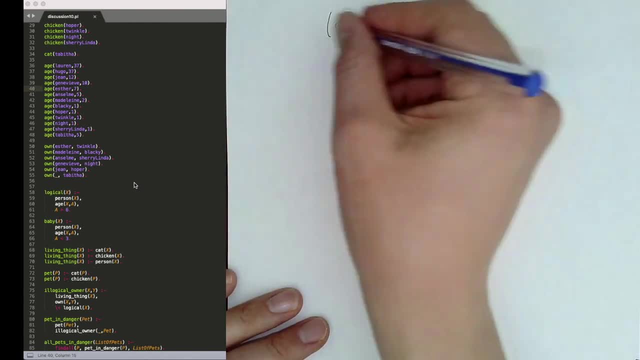 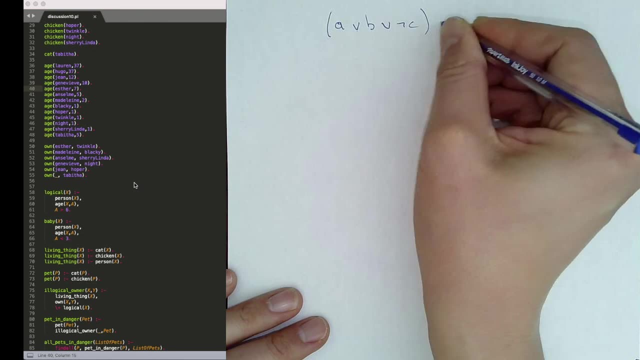 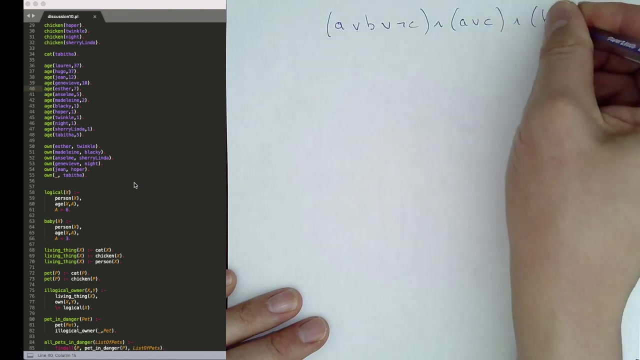 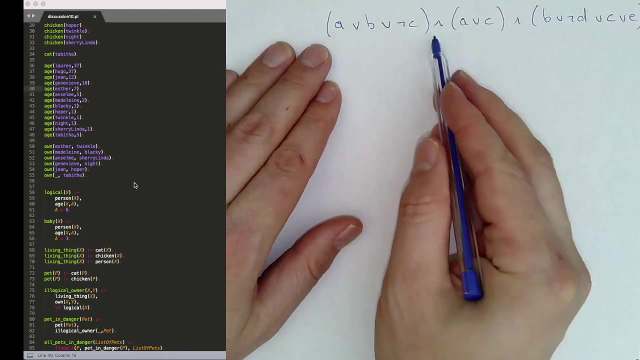 the closed normal form where you have a disjunction. so only ors like that say: you know A or B or not C, and A or C and B or not, D or C or E say something like that. So these are clauses separated by. 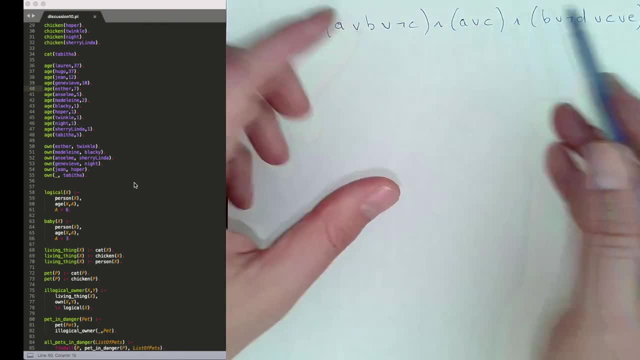 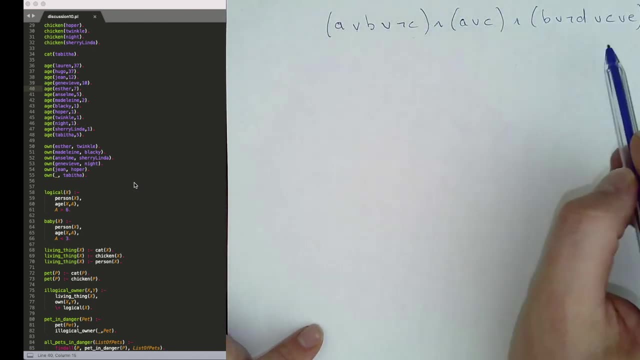 So clauses are only disjunction and they are all joined together by conjunctions, So and right. So you have only ors, within the parentheses, and and between. Anyway, you can translate actually any kind of proposition into a clause form, clause, normal form, like that. 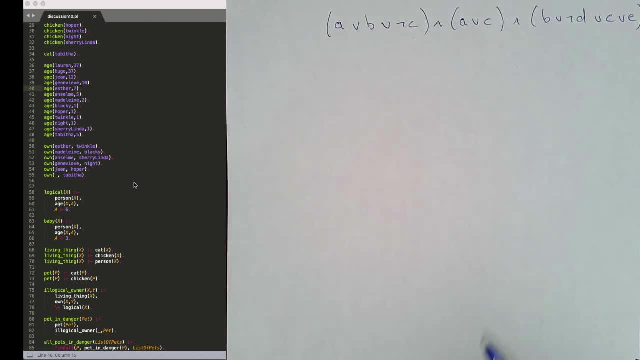 These are, in general, in general, very, very hard to solve. They are considered, They are considered to be very hard problems And this is something you'll see in in the course 475 in the top on the topic on complexity. So they are very hard Why? Because eventually, to decide what combination for A, B, C, D, E will make this satisfiable. 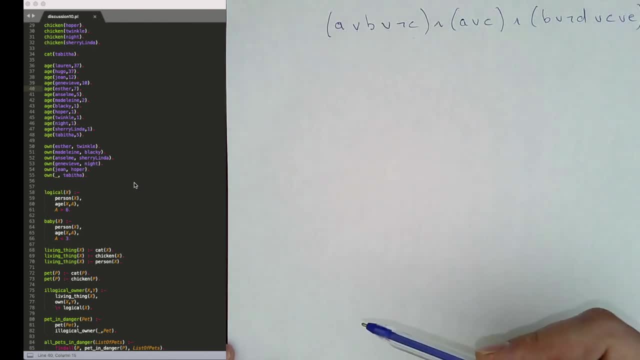 You have no other choice than just test all the truth values. So it's it's an exponential time to solve that You're going to have to test: A is true, B is true, C is true, D is true, E is true. 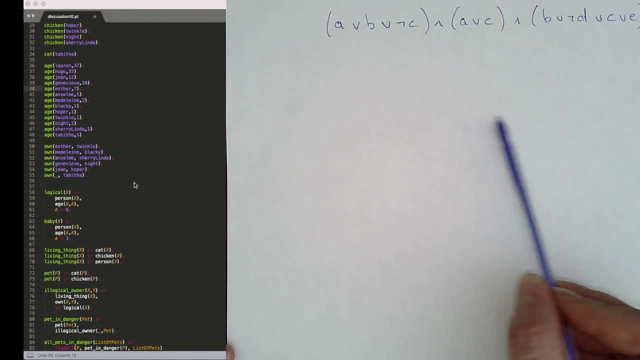 And then the same thing with E false, and then the same thing with D false, etc. And you have to test all kind of all possible combinations until you find something satisfiable. So in the worst case it is, it takes a very long time. 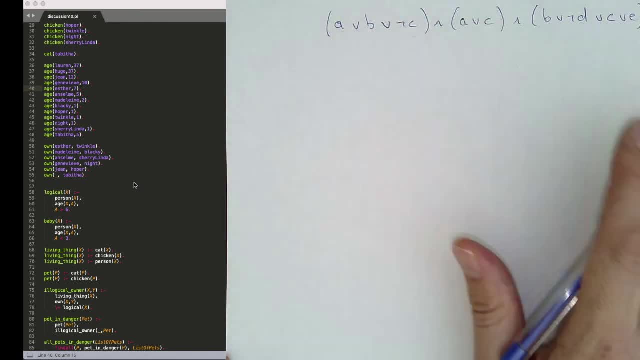 So I just want to mention that as a background. it is very hard to solve logical problems. Now Prolog does it in linear time. It's actually really really fast. And to do that they kind of put a constraint on what kind of formulas here are allowed. 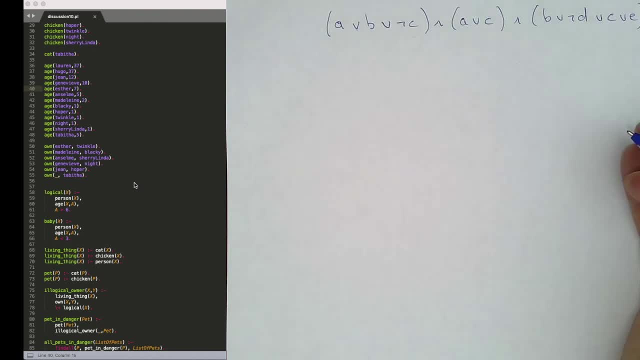 Only a subset of those are allowed, so that, so that it can be doable in- not in exponential time and in linear time And- and, as you can, your pre-experience Prolog is surprisingly fast actually. So we'll go back to that, But that was a parenthesis. 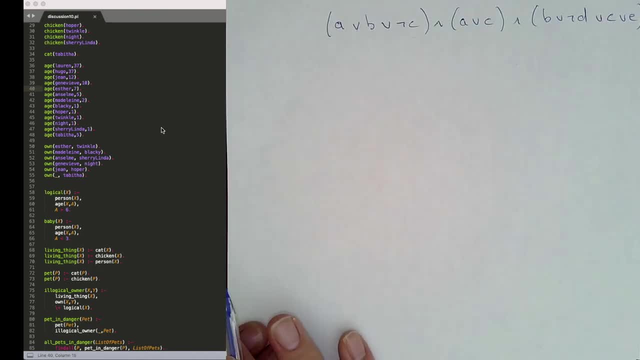 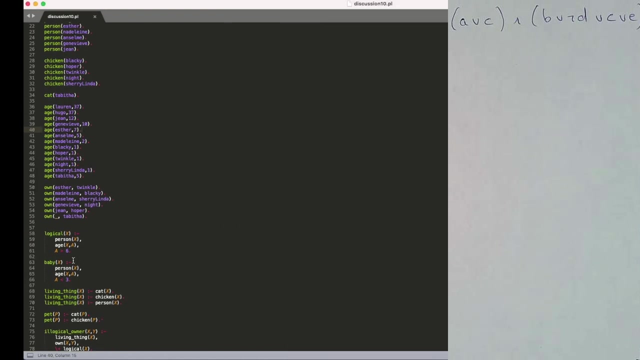 OK, so now let's do this. Let's dive a little bit into So. I built this, this tiny little program based on living beings in my household, including people and pets, And there are some, some facts here, some rules here, And we'll dive a little bit more into that. 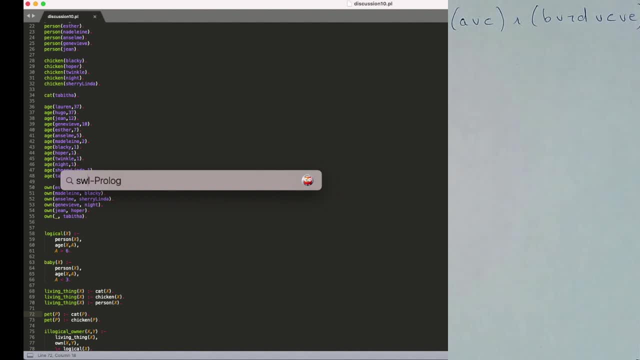 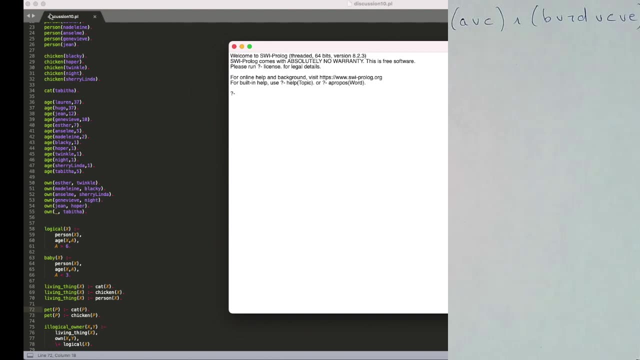 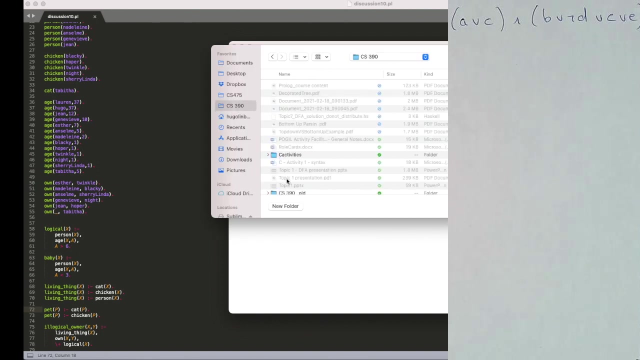 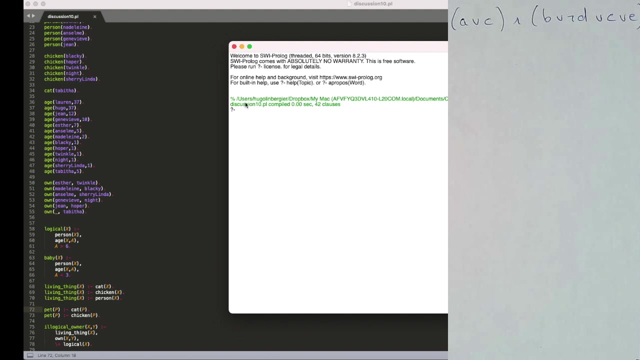 So I'm just going to dive in here, Sorry, And just start SWE here. So SWE is a standalone program. It's a standalone application. It's very easy to to use. I go to file consult to consult my, My file here. 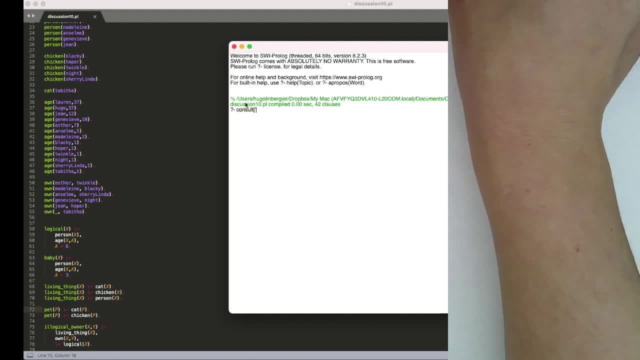 You can also use consult, Brackets, quotes and filepl. You know, I mean in the name of your filepl. I mean you have to put the whole path actually here and a dot here And if you press enter it's going to, it's going to work. 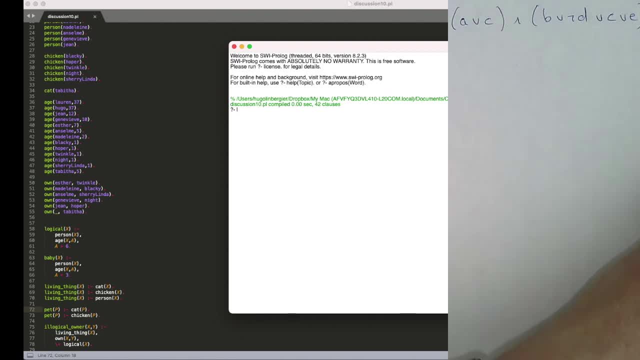 But you can also use the menu so I can ask you know who is logical in the household. Basically, you know who has the age of reason. I can ask things like you know what are the pets And? and I can ask you know. 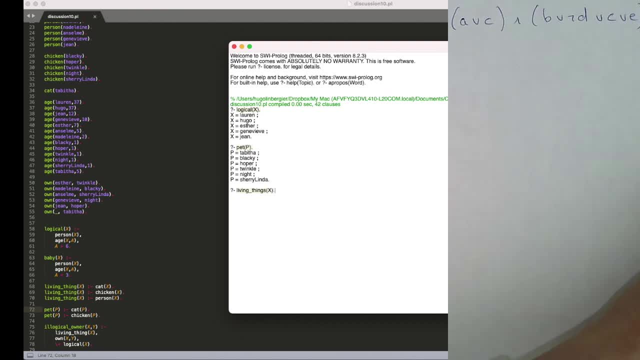 Living things As it's. So here are the living things. I press semicolon every time I want to have another answer And and I can ask a little bit more Completed things. you know I can ask, you know I can do. 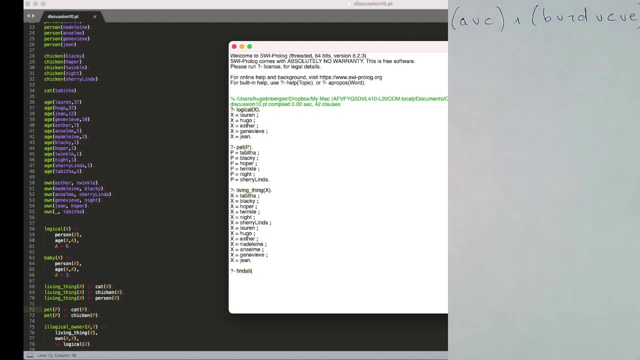 Use the find all built in query. They find all X, such that X is a living thing, and put that into the list of living things. And here is my list of living things. You can also query binary predicates. It means predicates with multiple, not just one. 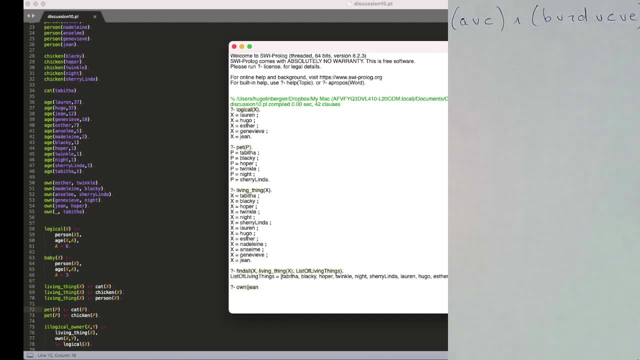 But multiple arguments Again, as you know, what does Jean? You know, oh, I can use the variable owned by Jean And Jean owns Hopper and Tabitha. OK, so that's, that's quite simple. You have tutorials. I suggested that can help you with this piece. 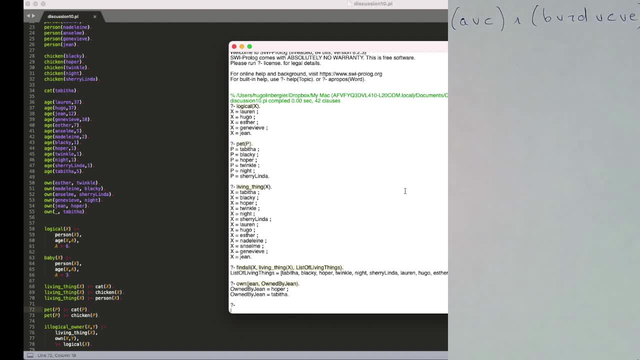 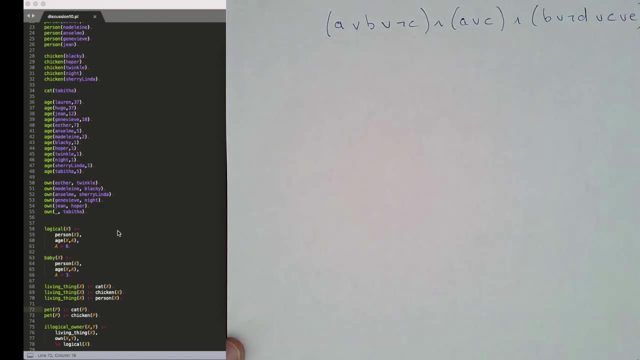 It's really not necessarily the focus of this presentation. What I would like to talk about is more how Prolog is organized here And what are these and how does this work? You know a little bit of looking under the hood of Prolog and logical programming in general. 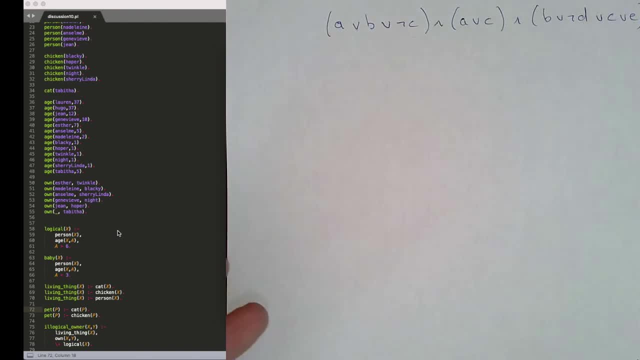 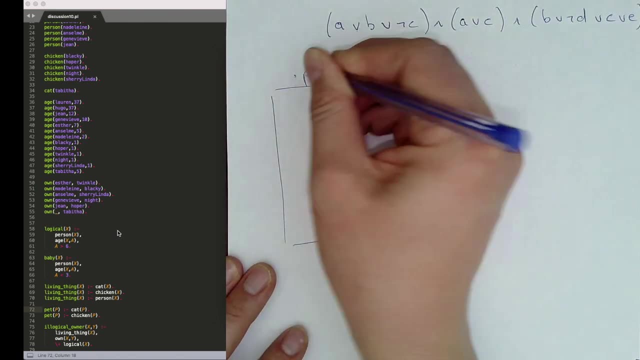 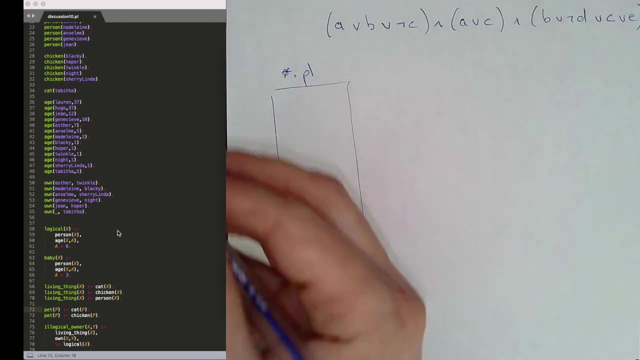 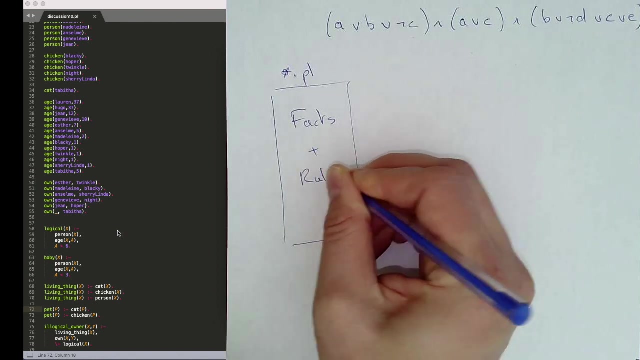 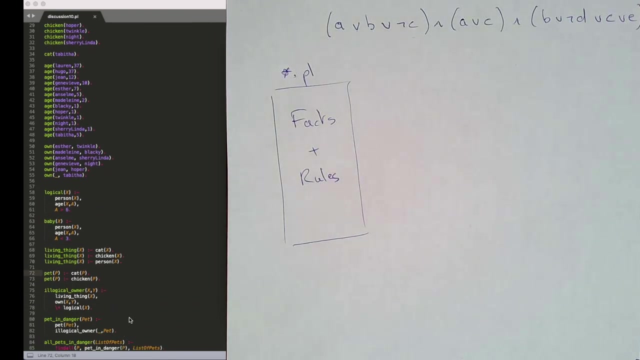 So Prolog, So it's basically consists in a program. Right, You have a dot PL file And this file is composed on of, you will notice, a series of facts and rules, And so you have here. the way I organize is I started with the facts and then I put the rules. 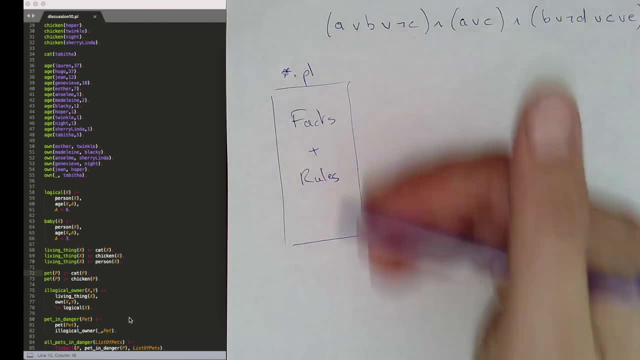 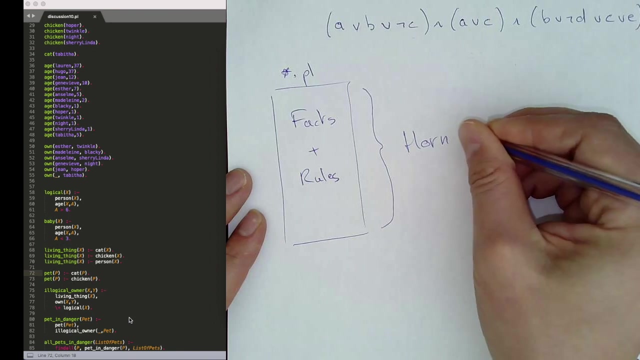 I could have done it differently. Of course there is no Really order here. I mean, it doesn't really matter, It's just for an organization point of view. And it happens that all of these facts and rules are whole, all what we call in logic on clauses. 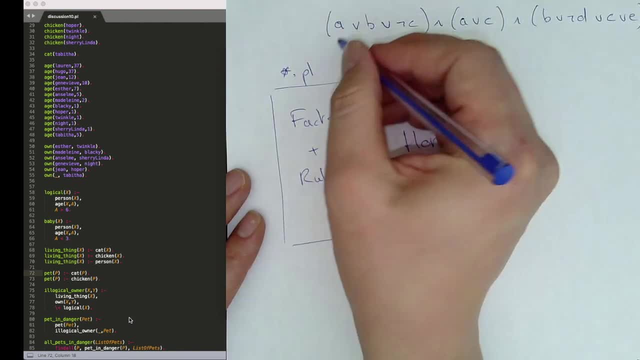 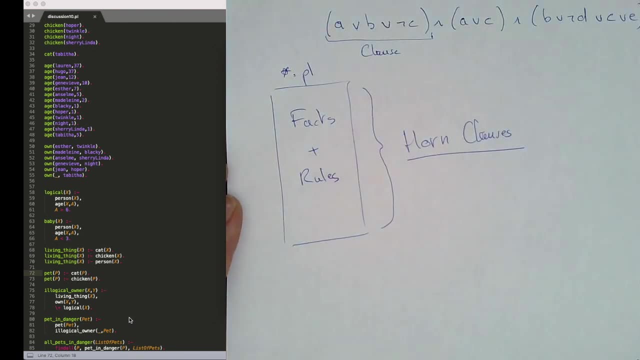 So there are a specific kind of clause. So I said: you know, this is, this is a clause. What is a clause? A clause is a disjunction of literals. So this is a literal, This is a literal And this is a literal. 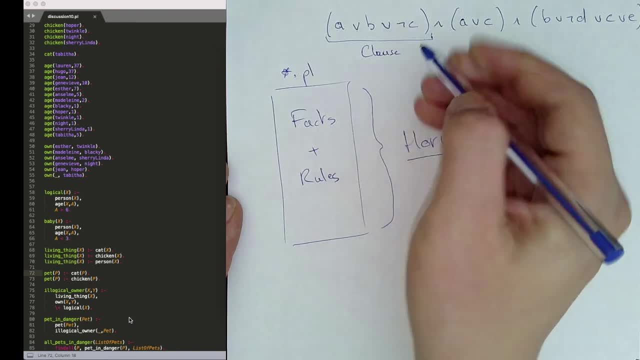 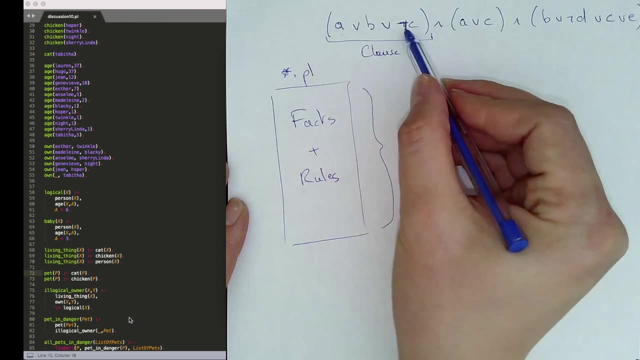 Right. The literal can be positive or negative. This is a sign of the negation, Right. So a literal can be positive or it can be negated. So positive, positive, negative. This is all positive, This is positive, negative, positive, positive. 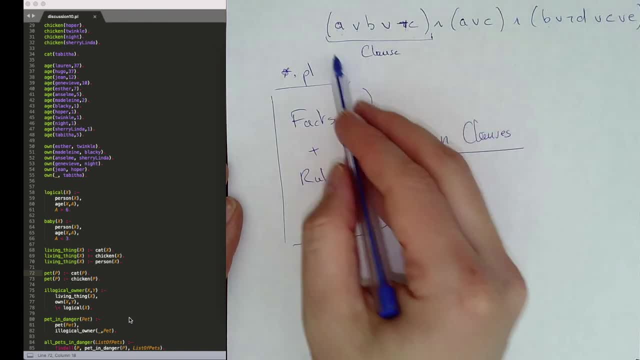 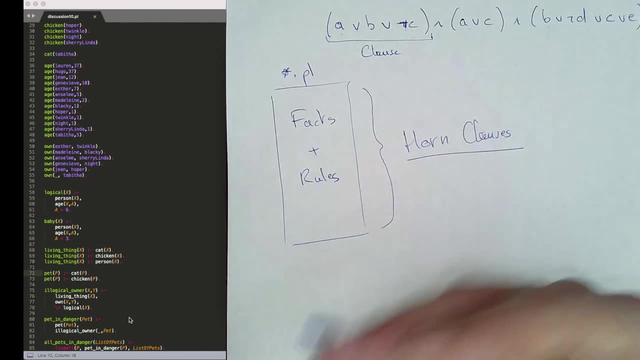 Okay, So a whole clause is a special type of clause. So clause is always a disjunction, It's only ors Right. So it's very poor, Right. You cannot express so much. I mean with just clause. you cannot express so much. 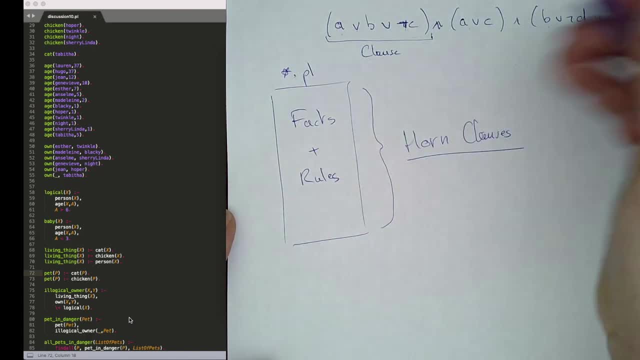 You need to put them together with ands so that they are more meaningful, But here our program is only composed of whole clauses. A whole clause is a clause that has zero or one positive literal, And we'll see what that means and why it's the case. 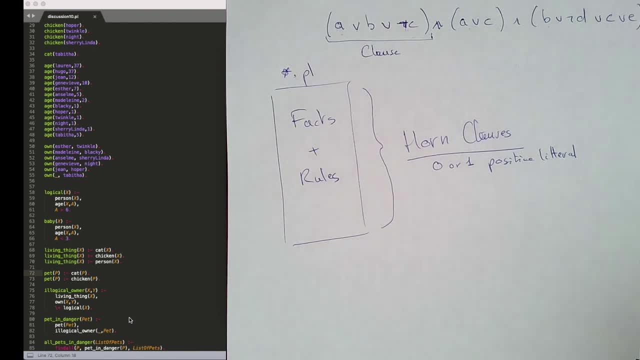 I'm just going to give you a little looking ahead. This is. the reason for that is that this solves the problem we mentioned before. If you have only zero or one positive literal- which is actually not the case in any of those- there is a way to solve the satisfiability problem. 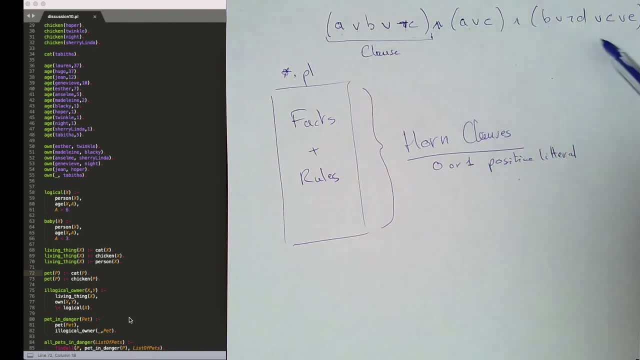 Right The problem, which consists in finding a solution such that this is satisfied. That makes it such that we can have a linear algorithm to solve it And therefore it's not exponential and not intractable. So that means that the solution can always be found in a reasonable amount of time. 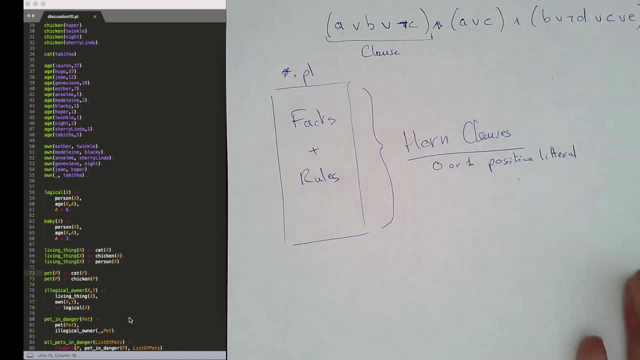 So we can find a linear resolution process for the satisfiability problem. So that's why we impose that condition: Zero Or one Positive literal, And we'll see a little bit more about that. Okay, So if you have zero or one positive literal, just let's take the case of one positive literal. 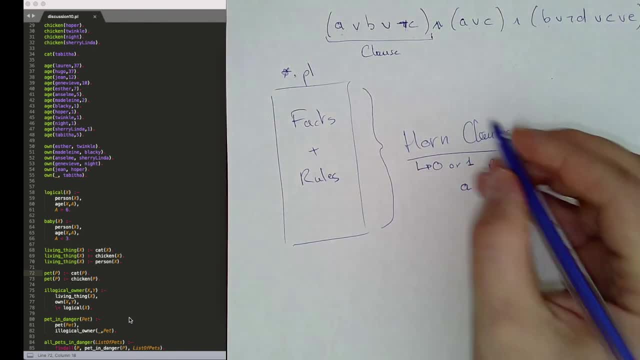 What does it look like? Right, You're going to have something like A or, let's say, instead of B here: A or not B or not C. Okay, And this actually can be, Can be Changed into, using the basic rules of logic, into A or not B and C. 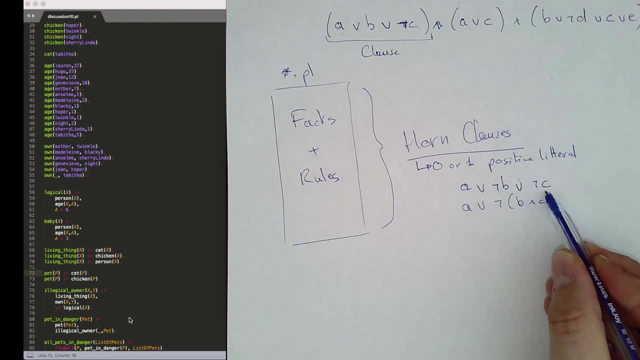 Because not B and C is the same thing as not B or not C. And we have another rule that says: you know, if you have somewhere you know A implies B, It's the same thing as not A or B. It's something really convenient to know by heart. 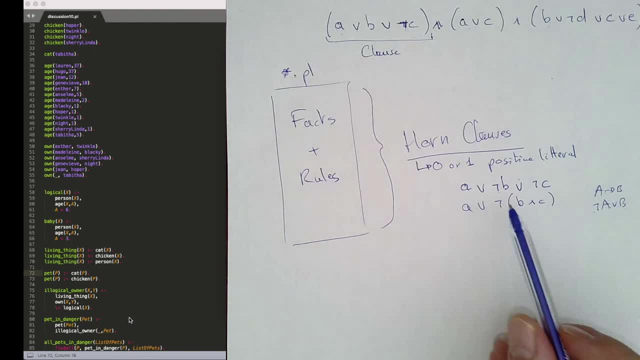 A implies B is the same thing as not A or B, So here you have not B and C or A, So that means you could actually replace that by B and C. Sorry, And C- This is the end- Implies A. According to that rule. 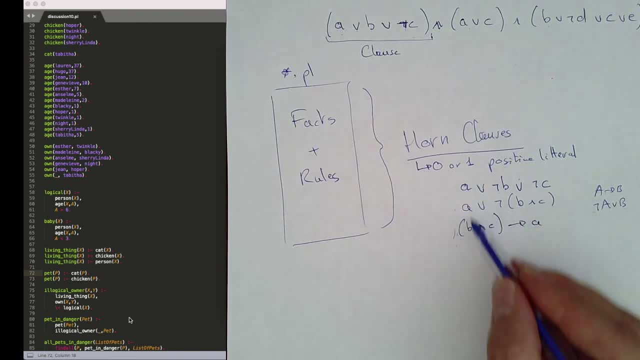 This is the same thing as this Right. So all of these are the same thing. And now let's invert Right And write the arrow the other way around. So instead of saying B and C implies A, Which again is the same thing as this own clause. 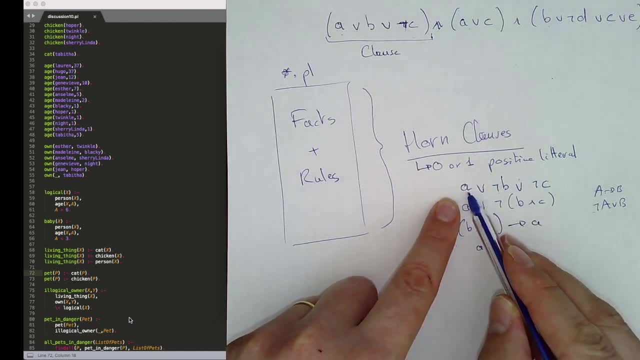 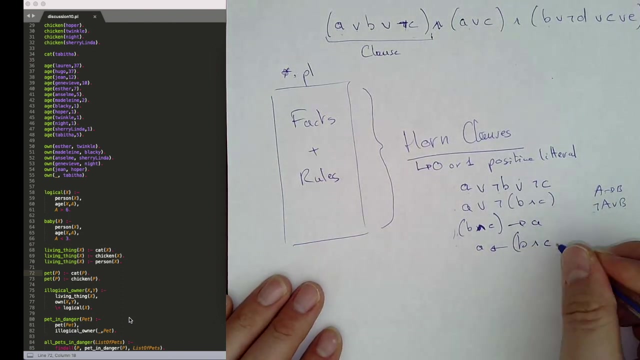 Right, That has only one positive literal and two negative literals. Negated literals- Right? Instead of saying B and C implies A, I'm saying A is implied by B and C. Right, It's exactly the same thing, Right? I should keep the parentheses to make this clear. 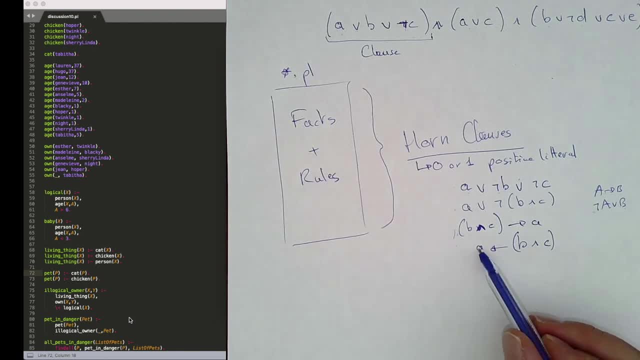 They go together, And or you can say A if B and C, B and C Same thing, Right. If you say A is implied by B and C. Or you can say A is true if B and C is true, Right. 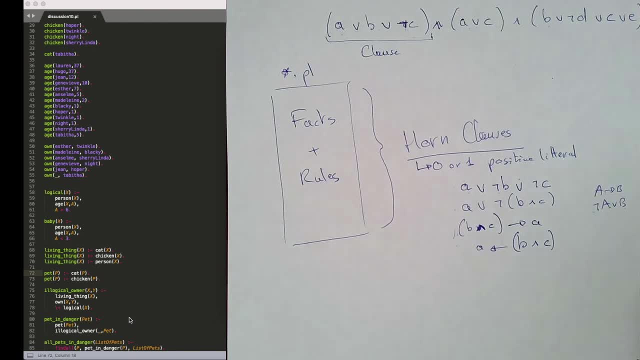 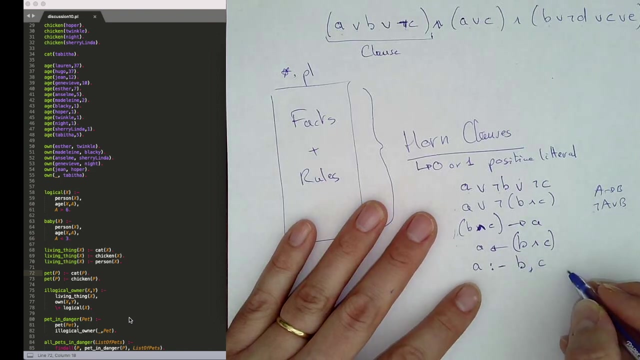 It's the same thing. And now we have basically here our prologue schema, in some sense I mean pattern, which is going to be A, the prologue neck, And then we replace the end here by commas B, comma C. So when you have in prologue, like here, you know logical X with the neck. 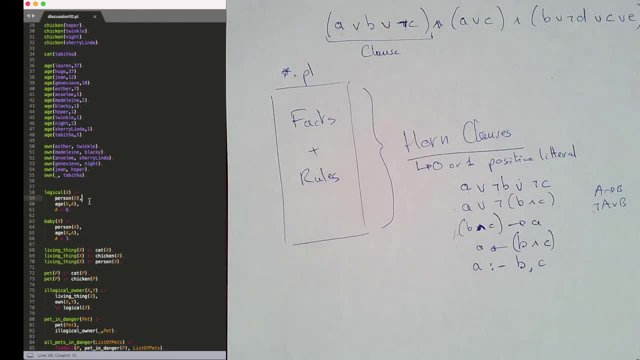 And then a list of propositions. This is really what this means, Right? This means, you know, if X is a person and A is the age of X and A is greater than C, Right? Then X is logical. So that's how you can read. 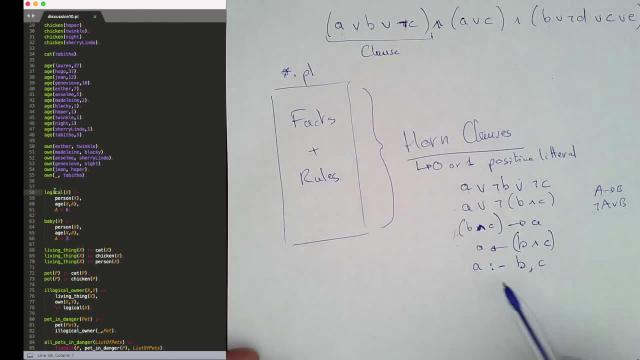 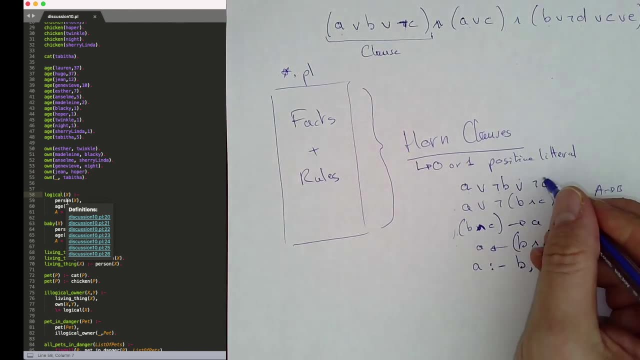 I mean it's convenient to see that because that's really the meaning of these prologue rules And that's how you can read them. It's not really convenient to read them as horn clauses, because this is not as intuitive to say A is true or not, B is true or not, C is true. 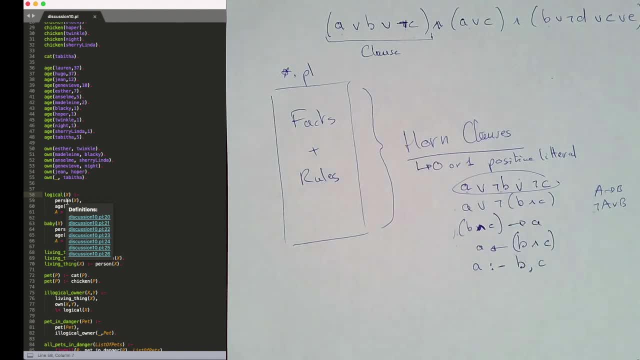 It doesn't like cognitively doesn't have the same, It's not as clear in our mind. Then, when we say B and C implies A, This one is the most. I would say, this one is the cognitively the most meaningful for a human being. 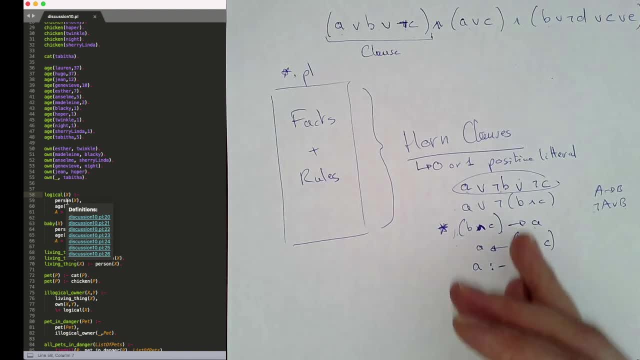 So that's why also prologue uses that one. It's not just because horn clauses are convenient for resolution perspective, but also because it actually is easy to read, Right, So you can either read them, read here. You know the way I did it. 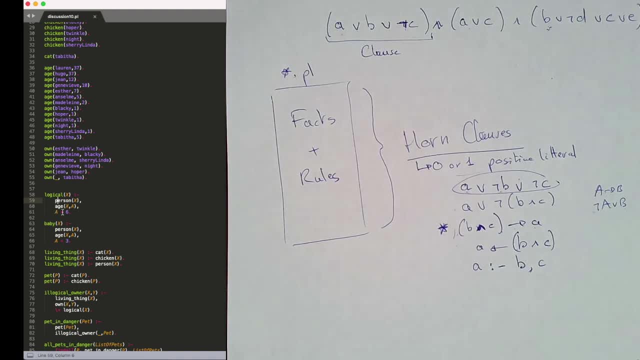 You know, if X is a person and X is, I mean A is the age of X and A is greater than six, then X is logical. Or you can read them linearly the way it's written in prologue, which is: X is logical if X is a person and that 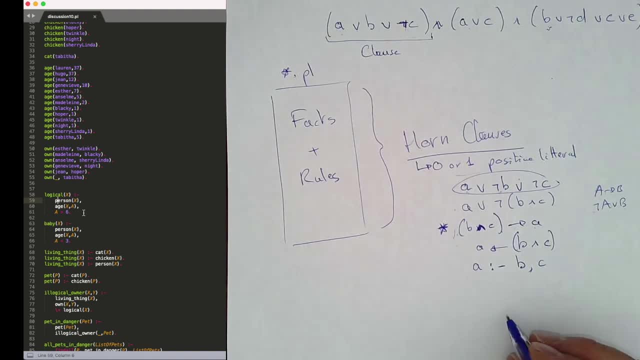 OK, So. So, So these, these are basically just horn clauses. Right, These are all horn clauses Because they always have one positive literal And then negative literal, And we'll see. we will see why one or zero and why not two and more. 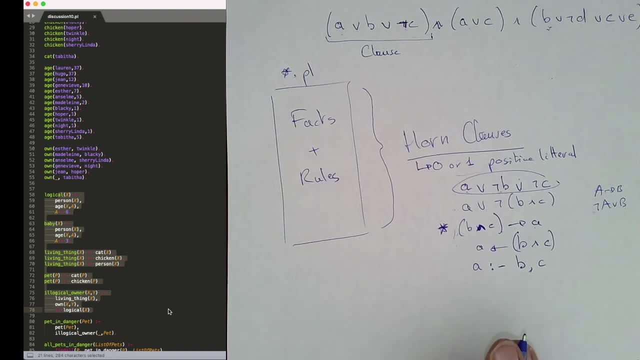 But just just so we clear on the terminology. So I call this: This is the neck, The prologue neck, This is what we call the body And the head. So you have the head before the neck, Which is kind of. 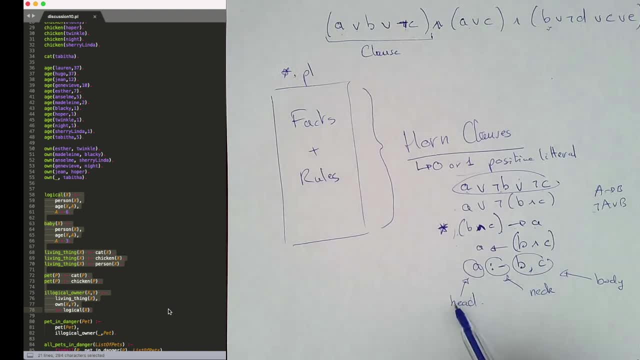 Kind of makes sense. The neck and the body. It's kind of a good. It's kind of it kind of makes sense because You notice that the A, what ends up being before the neck When I did my transition, is the only positive literal. 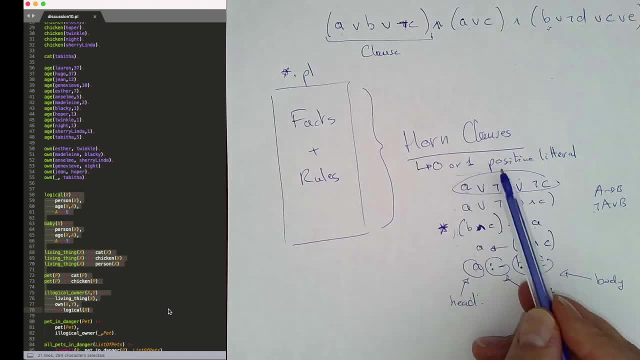 Right Because we cannot have more than two, more than one, We are at most one positive literal. It kind of makes sense just to call it the head, Because it's unique. Right There's only one, always on the left of the neck. 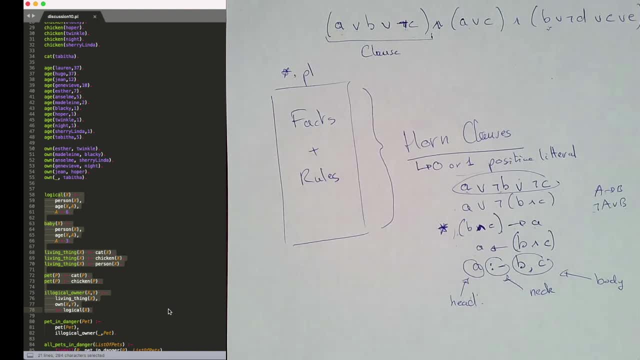 And then on the right, You can have a list as long as you want. Right, There is no condition of the negative, Negative literal, So you can have as many as you want. Right, You can have very long rules, So the body is is plural. 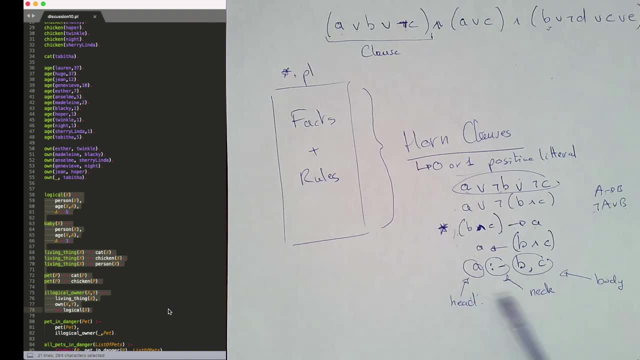 And the neck is unique. So it's kind of it's kind of a real neat terminology And this is a neck. So OK, Now What about the facts? Right, We have facts here. Facts, They don't have this. 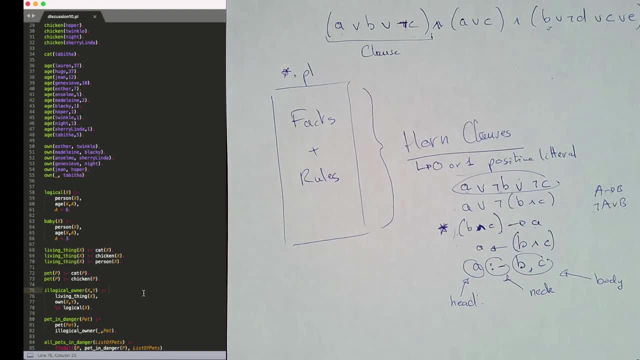 You notice they don't have this, This shape. Let me write one of the one of the rules here, just so we can see more clearly. So I say logical X. So we have here the head, and here I use only what we call propositions. 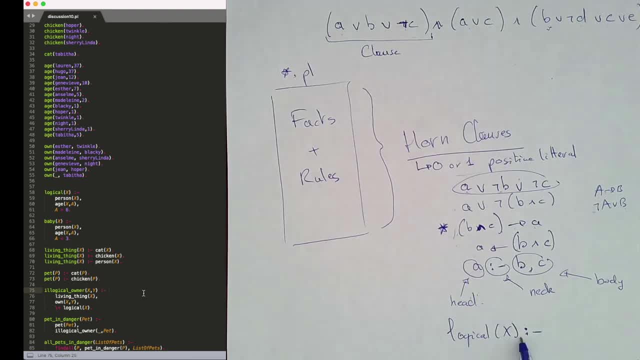 So they are just true or false. Here it's the same thing. Right Logical X is true or false. Now, this is. this is not just. It's more precise than what we call proposition. logic is what we call predicate logic, because a proposition is not composed of a predicate and a subject. 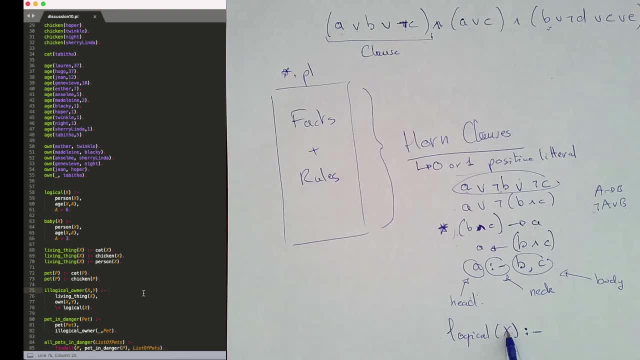 And it is true only if the subject falls under the predicate OK. So it's just a sort of How to say that Enrichment Of Of this Right With with more details if you want. OK. So here is our example- was. 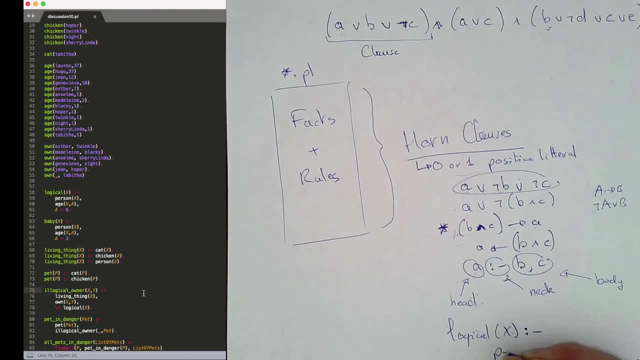 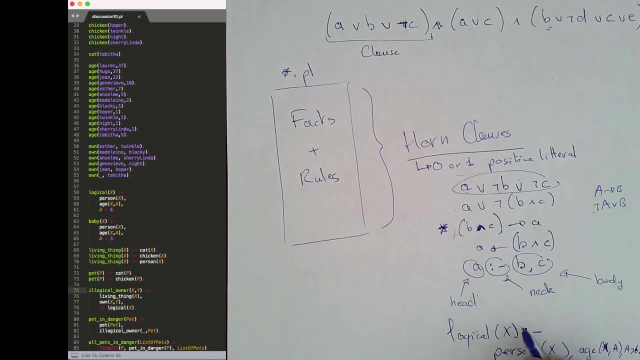 Person X. And so you have here Again The head, The neck And The body. I put the body here in one line, but It's fine to put it in several line in Prologue. The prologue is the same. 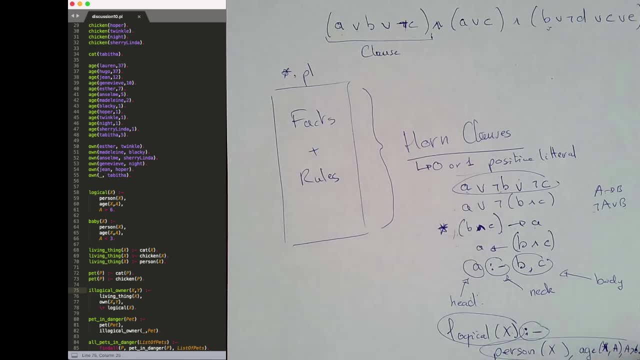 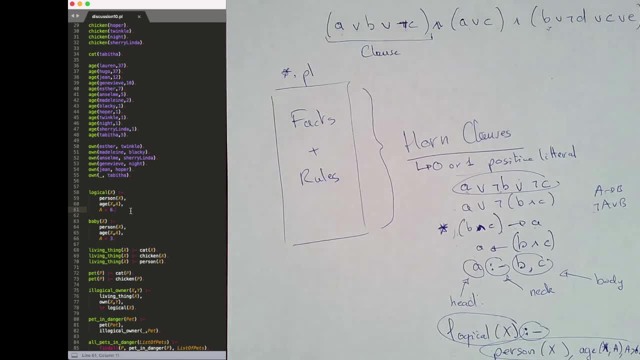 It's the same, It's the same, It's the same. The prologue is very, very Permissive in terms of the way you organize things. It's only the punctuation that matters. Talking about punctuation, Do not, Let's not- forget the dot here. 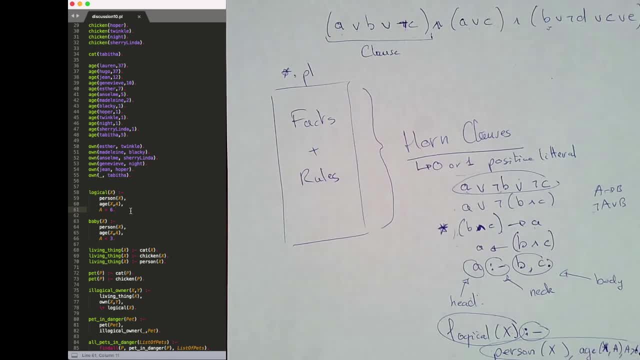 That ends- I forgot it here. That ends our Horn clause Basically, Right. So A program here is going to be a set of horn clauses, Right, We have here several Rules. We have one rule here Another. 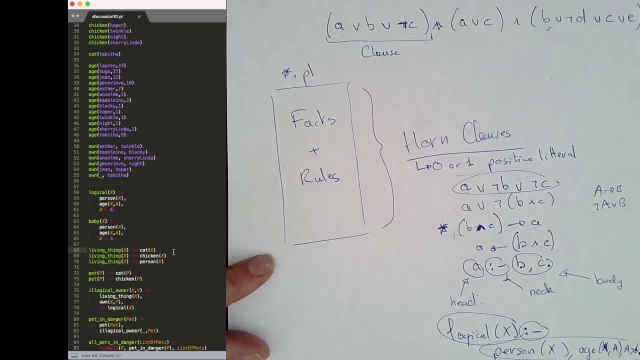 another one, you know here. here I mean, we have multiple rules, right, each rule is a whole clause. so basically the dot is separating each own clauses, just the way the end separates one clauses here, right? so our program is not going to be just one one clause, which would be very weak in terms of expressivity. it doesn't mean. 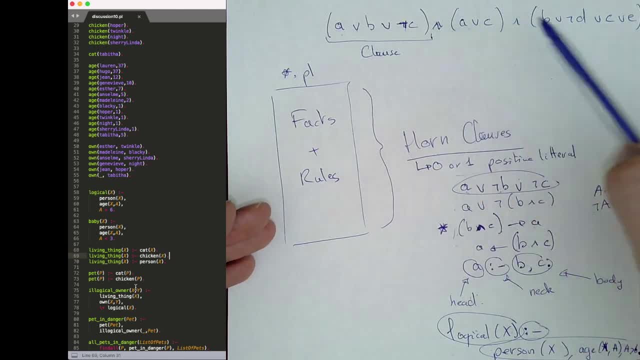 much. I mean you cannot do much with it. it's a set of one clauses separated by dots, and they are basically all they all have to be true. so that's they are all separated by and to constitute what we call the closed normal form that basically has the same kind of expressivity power, expressive power as 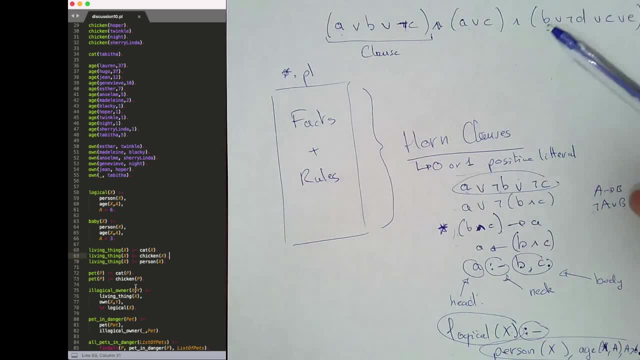 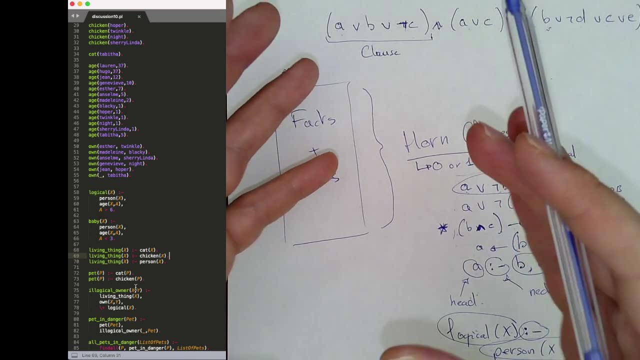 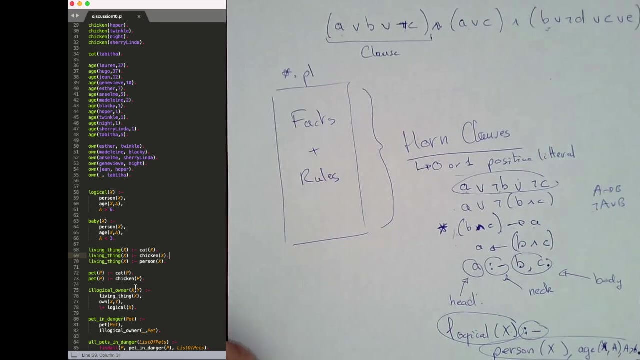 as logic in general, where you can have and or implication and stuff. so. so the dot is separating all the. all clauses are brought together by as, as, as conjunction, basically okay, so these are the rules. now we can ask: what about the facts? well, the facts- I'm gonna just write one from from here, you know, like 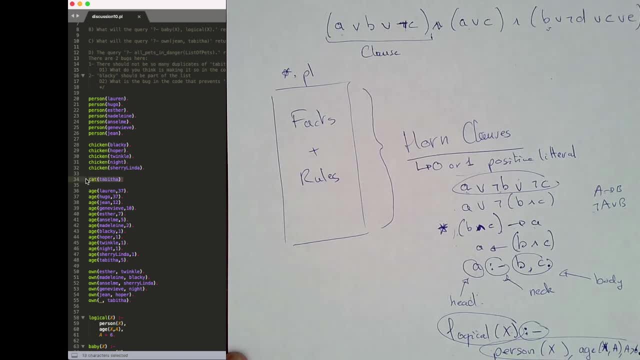 we have the fact that Tabitha is a cat, for instance. it says here: so cat Tabitha is a fact. and well, this is actually also a home clause, except it's one that has no negative literals. um, no, sorry, that has no. let me rephrase that it is one that has nobody. so, yes, no negative literals, okay. 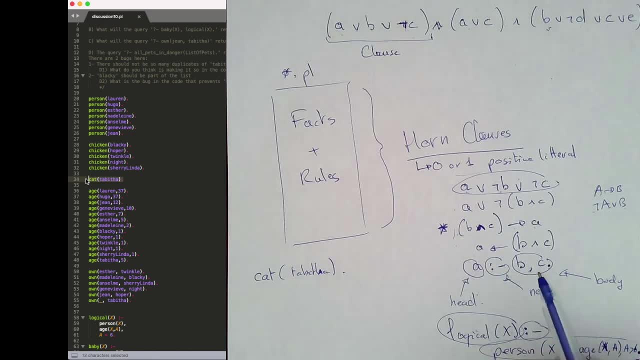 so you basically have not, don't have the part after the neck, so you don't need the um. uh, it's just a head right. so if you translate that, if you follow the same um, this is this is basically just the a right um. a is true, a is true. you know. a is true. a is true. a is true. you end up. 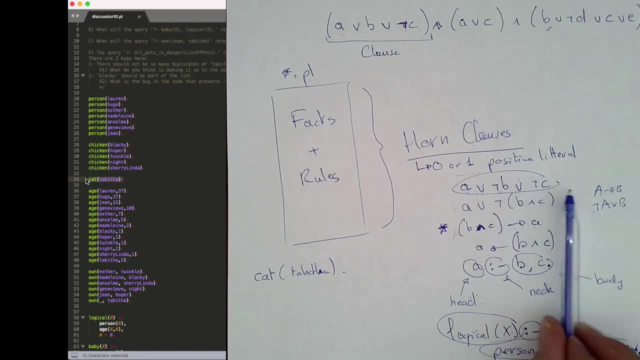 with here, without the b or you know, the the, not b or not c, so you end up without this p, so you just have a. so you have the head without the neck and the body right, you still have the dot at the end, very important to separate from other clause. that's what a fact is, um, you're just saying 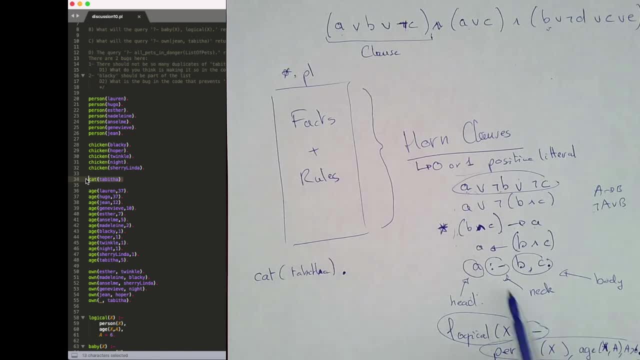 tabitha is a cat, that's, that's a fact. so it's, it distinguishes it from the, from the rules. so again, this is, this is the head, and there is no, there is no body. so these are headed horn, horn clauses, these ones and these ones, the facts and the rules, because they have one positive: 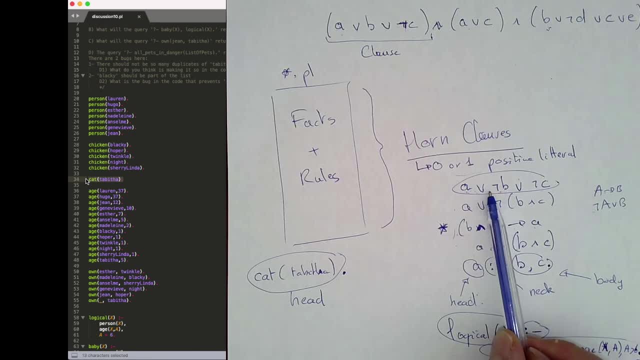 literal and possibly zero or any number of negative literal. if it's zero, negative literal, it's a fact. if it's one or more, it's a rule. um, this is what we call a rule. now we say that a horn clause could possibly have zero positive literal. that means zero positive, that means they have no. it has no, no head that's. 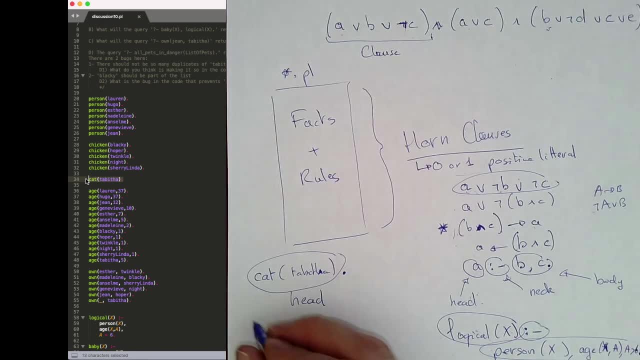 what we call headless clause. right, so what would a headless clause look like? well, a headless clause would be basically the neck with no head, no positive literal and only negated literal on the right right. so it would be, you know, b, c, d, e, for instance. right that you have. 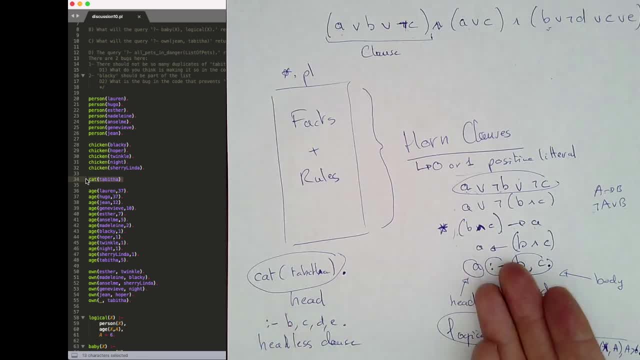 just a body and a neck and no head. so in terms of horn clause, it would be this. one would be, you know, not b or not c or not d, which is, according to a definition of horn clause, perfectly fine, because the definition says you have either zero or one positive literal. here we have zero positive literal, um, so that's, that's. 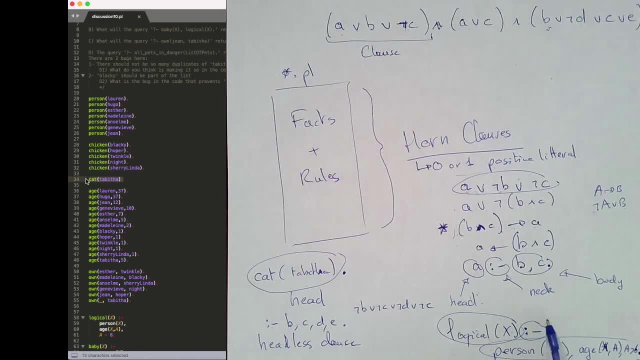 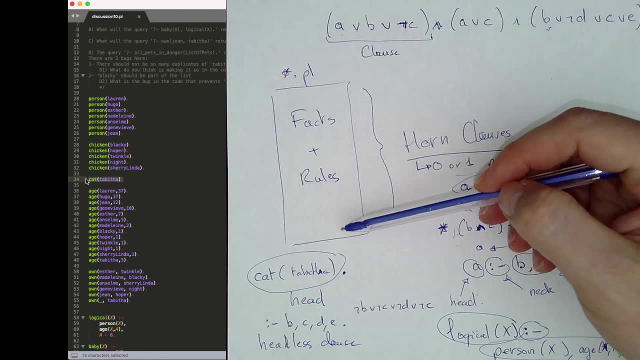 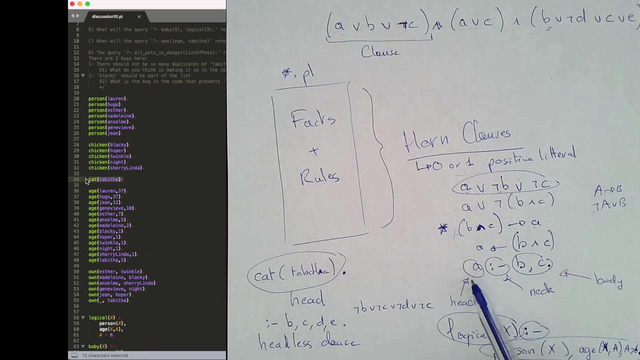 perfectly fine. and we have four negated literals. uh, where do they fit in this picture, right? so, um, uh, so, just the same way that you can read this as well: it's the head, so there is no body, so there is no if condition. right, it's not a. if b and c, it's just a. is true, right? cat tabitha is a cat, that's just true, there's. 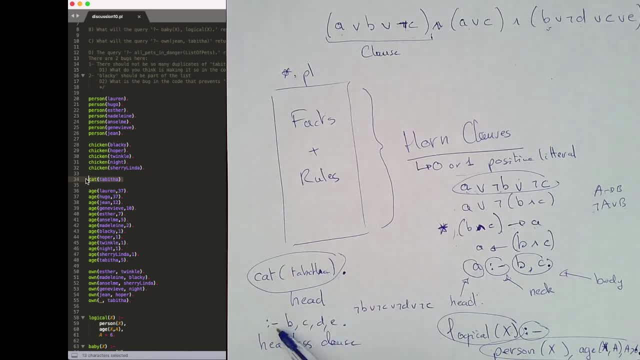 no condition for it. here it's kind of the opposite. it says i'm giving the condition for what? uh? well, what is important to understand is that a prologue. if this is a prologue program, what completes it is a another piece that is important to not forget. that is, the queries. 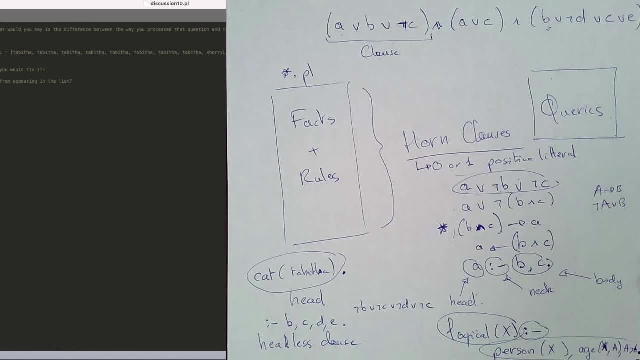 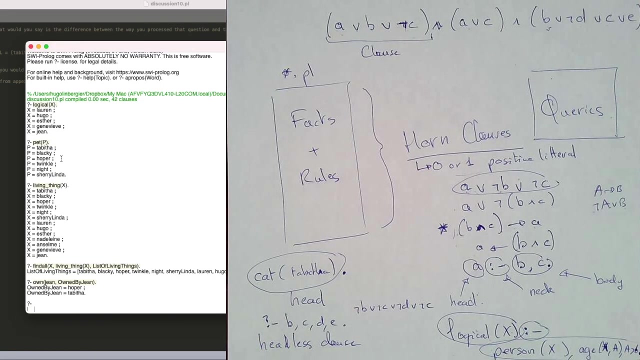 and the queries: are these headless clause, right? so basically, if you replace here the colon by a question mark, you have here the symbol that we have on sui here, right? uh, question mark dash to uh that ask us for a query. so when i put question mark dash, pet p, i am basically giving to prologue a headless clause. 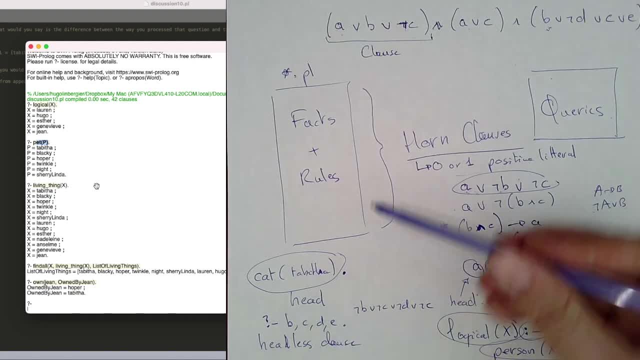 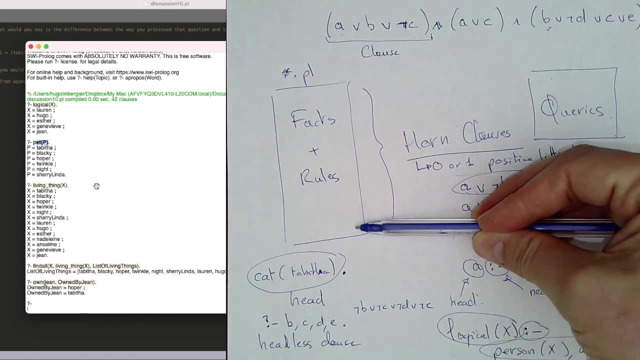 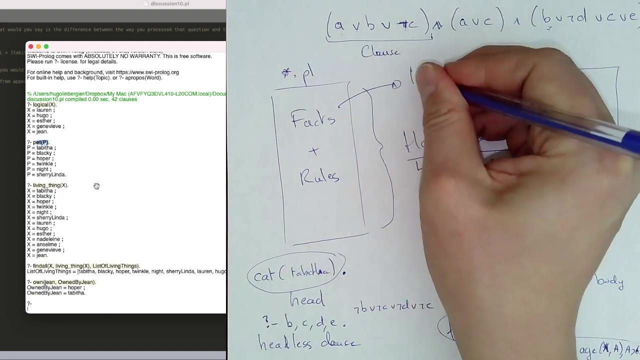 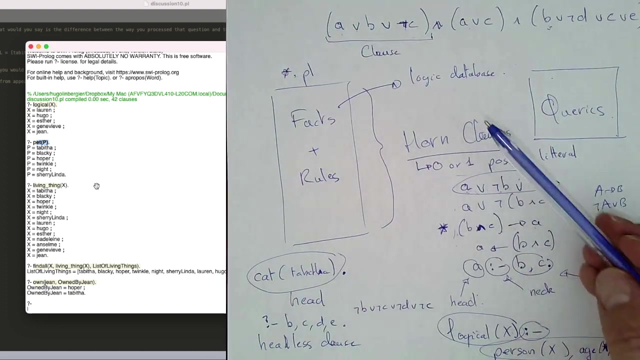 that is going to be checked against the whole logic database. okay, so, um, um, so that's um something. i wanted to mention that. this is our logic database, okay, constituted only of this kind of headed clothes, right, and query is going to, uh, the log, the query is, um, going to be checked against the logic database with one of these, um. 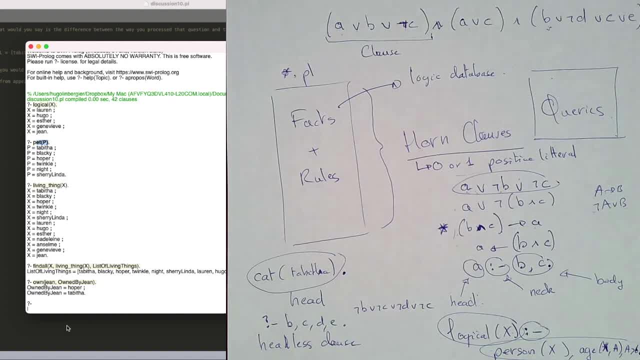 headless clothes. so you basically are going to, you know, like here, going in the queries or the logical data base, right, and you're basically calling this one. calling this ends in something else, not a puzzle you could might also use for some type of header focus. okay, and because the query is going to be checked against the logical database, like here, the logic dat Digital Y errand of militance, along with the logic update of cama code, is going to be among these quantities listed in this one. тогда, 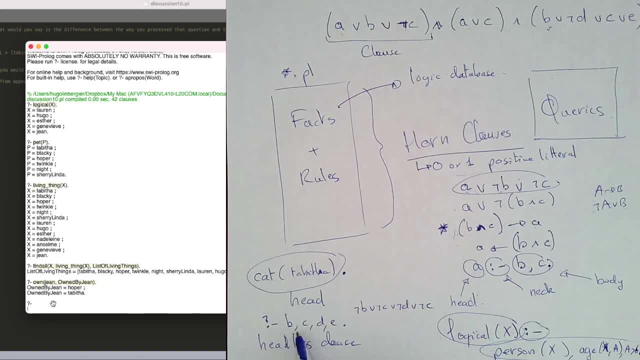 like here, going in a query is always consisting of a series of of literals that look actually positive but the way they're going to be translated is like they will translate into negative literals, because that's that's what they actually are, essentially right, and and the the query is going to be checked against the database to see if 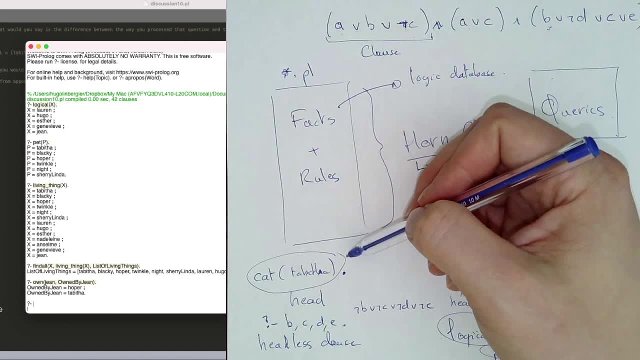 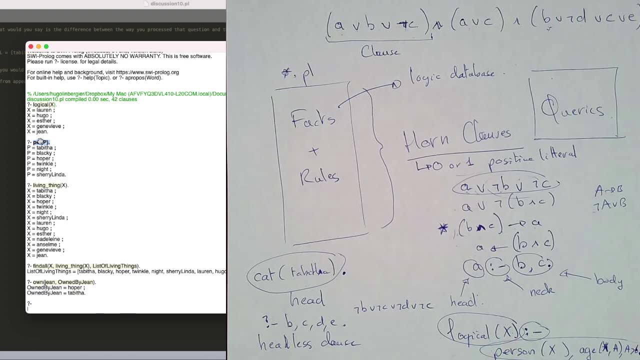 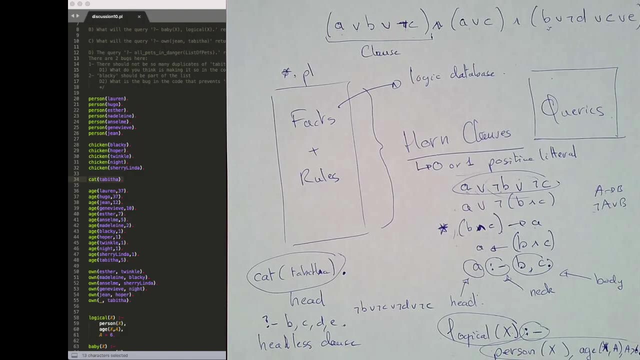 it is satisfiable for some instantiation of the variables you give right. so here, when we say pet, p, what prolog is going to do is going to check, and that's what it did. what are the instantiations of p that make this true, given what we have in the current database? okay, so, so. 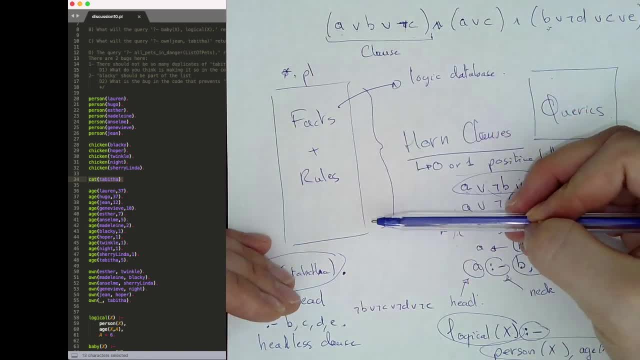 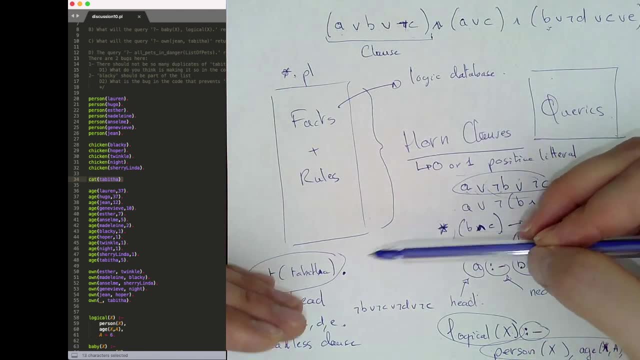 we. it's important to understand that prolog it's both a program, a dot pa file that is our logic database, considered facts and rules, and the queries. the queries are important. the program in itself is, it's a knowledge base, but it's not. it's not going to run on its own and that's that's a. 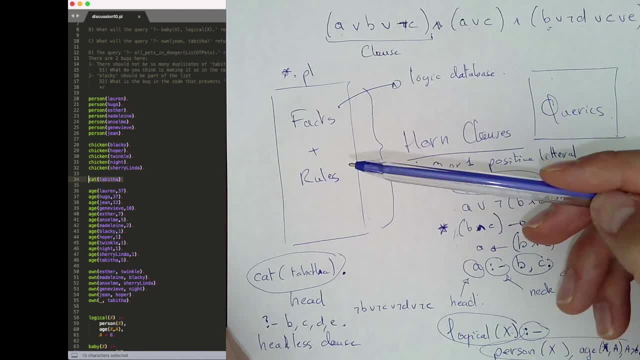 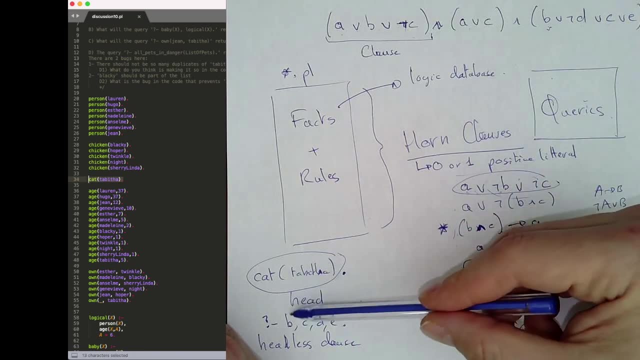 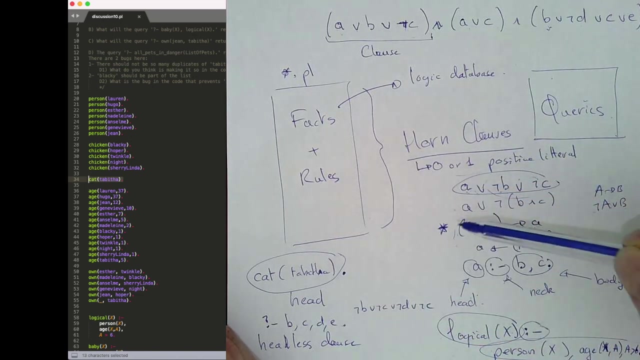 very important piece to understand right. you cannot just execute the prolog program. it won't do anything until you actually query it. so this close complement these and together they can be. they can. they can execute a satisfiability request. to check, is there a way to satisfy these? and because we are only limited to home clauses, it's. 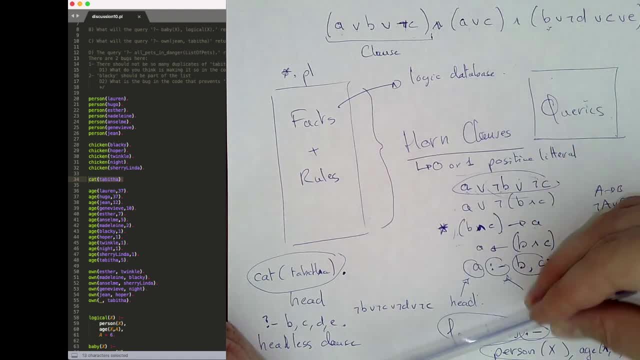 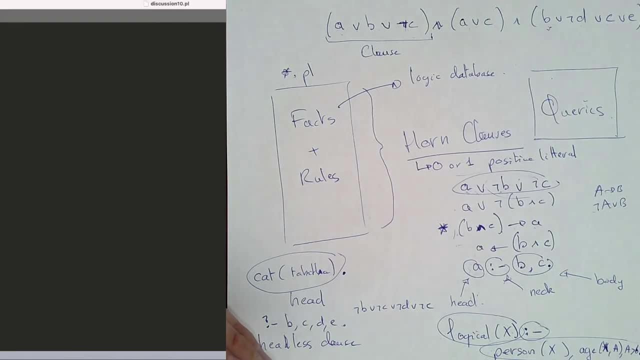 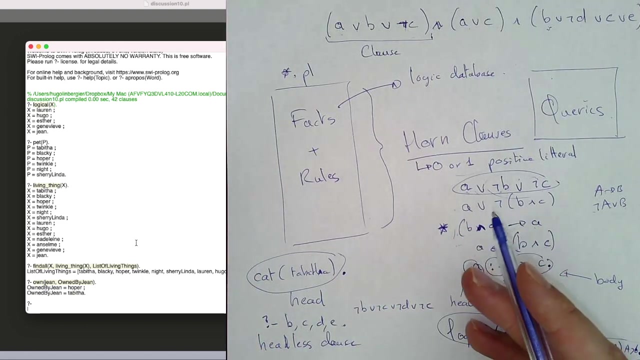 much, much, much easier and we're going to try, i'm going to try to give you a little taste of of how it works, how the process works, without getting into the details but um, uh, basically, and to give you an idea of of what makes it kind of of linear right. so when, when i ask uh to prolog, 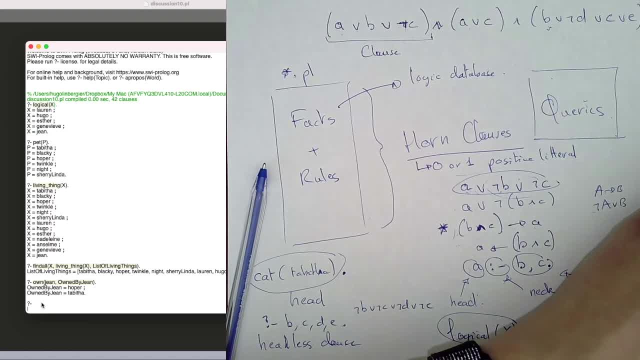 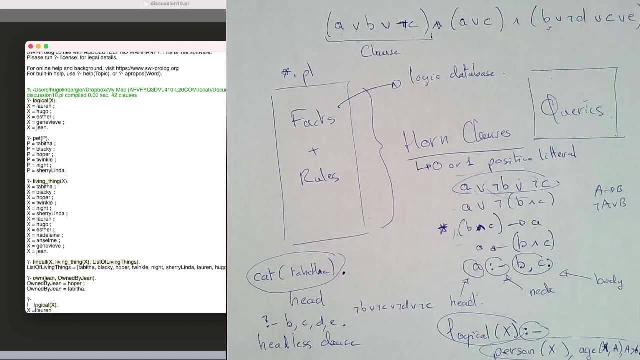 you know what are the the logical, the logical things. um, oh sorry, it's not working properly. okay, logical x. it gives me x equals lorin. so how? how is prolog solving this? um, this goal and and actually, the headless clauses? we also call them goals, so it's considered as a goal to be satisfied. i want to. 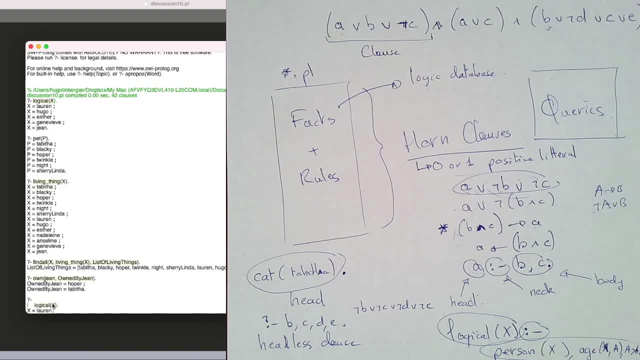 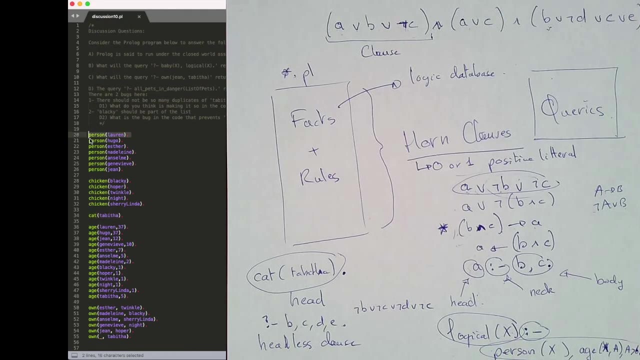 satisfy x is logical- logical being x being a variable. so i'm going to find some instantiation of x that make this logical true. so the way it's going to work is that prolog is immediately going to look in the database and really like index database, it's just going to go line by line. i mean home clause by 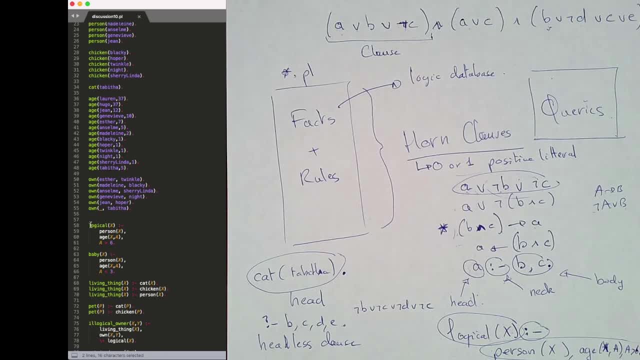 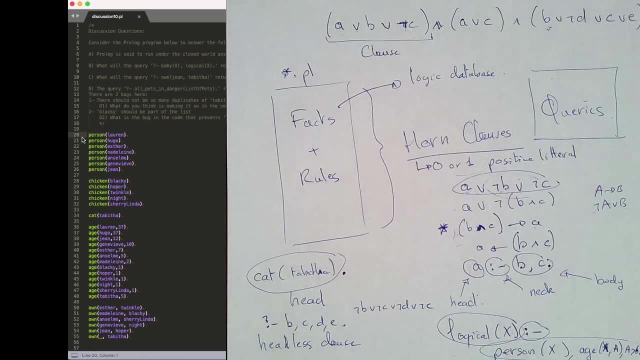 home clause, which you know it's not necessarily line by line because this home clause is on multiple lines, but it's going to check each one on home clause- sorry, facts and rules is indexed and it's going to take the first one that has a predicate logical right. so these are not the 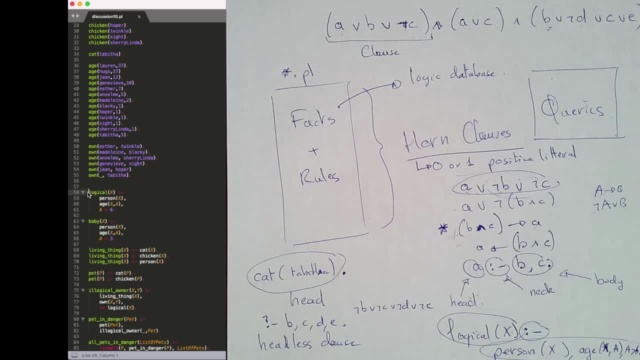 predicate logical, so it's going to stop at line 58. this is a predicate logical, so now that is the goal i want to satisfy is logical x. so if i had put actually some other variables here, that would have been more interesting, because now it would kind of 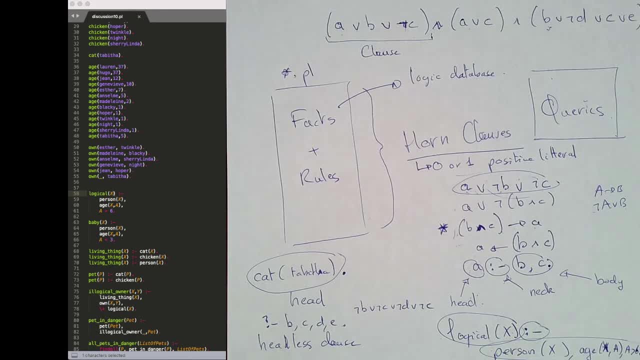 unique that variable. let's say y with x, and now let's satisfy logical x and um. the way it works is that now it's the, the goal is transforming to three sub goals: one, two, three, and these three sub goals are going to be linearly, one by one satisfied. so first i'm going to try to satisfy person x. 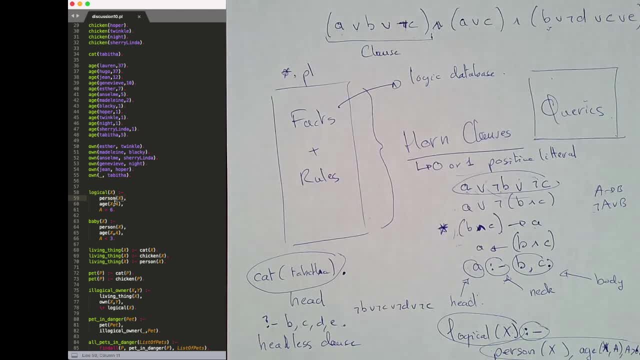 so person x becomes my goal to satisfy. so, um, you know, if i, if i put person x here, it's, it's going to also work exactly the same way as what it does when person x is taken as a sub goal to satisfy. so what does it do? well, again, it goes back and really, 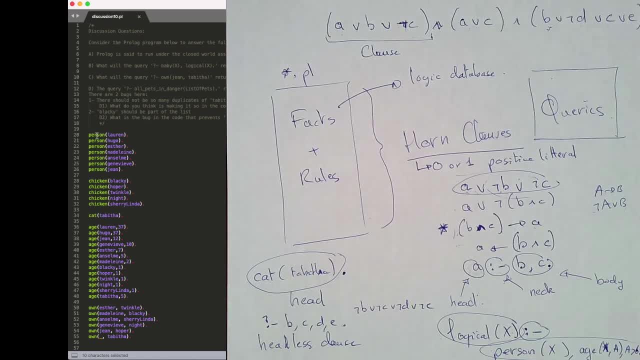 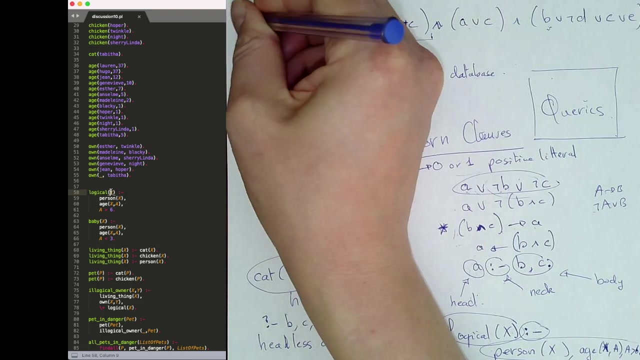 that's. that's how it works. goes back to the beginning of the file and look for person x. well, actually, the very first fact is the right predicate: it's person. so lauren is a person. so now x is what we say, unified with lauren, right? so we consider, the prologue is considering, x equals lauren and it's not yet validated. we're 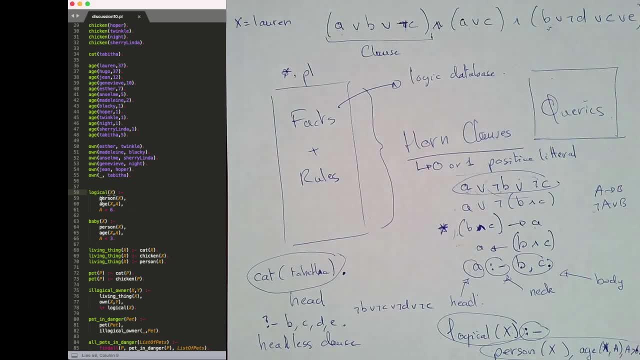 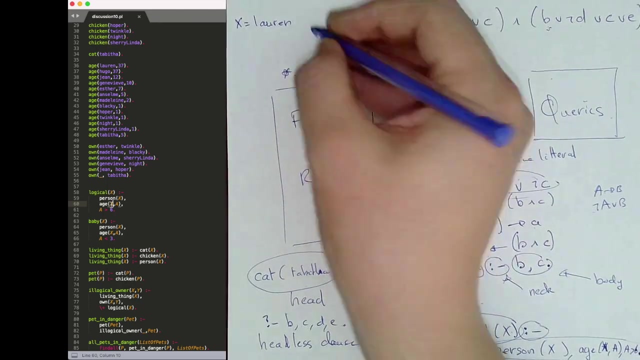 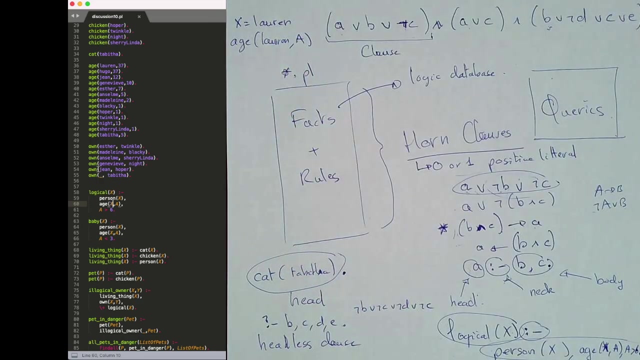 not yet there where it displays x equals lauren, because it's not finished, right, but it's satisfied. this predicate now age x a is, is going to. now we have x is unified with lauren, so it's actually going to look for age lauren a. so same thing goes back to the beginning and it's going to stop at line 36, age lauren 37. so 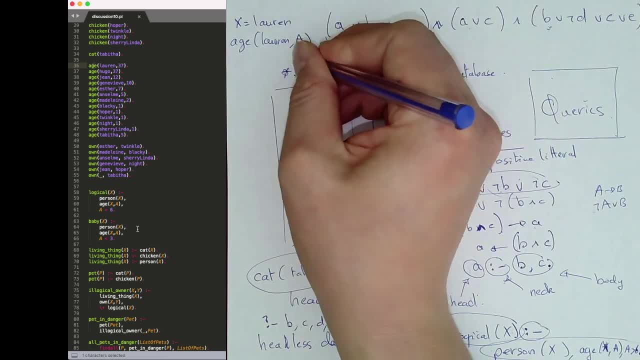 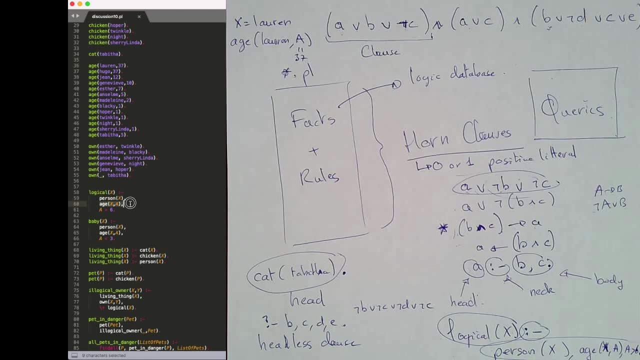 a is going to be unified with 37 right and um. and now uh, this goal is successful. these two goals have been successful. right, because we found a way to uh, to unify variables. that makes it successful. and here we don't even have unification to do, because a is already defined. 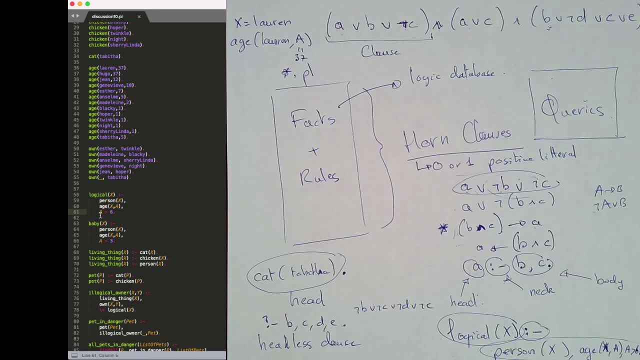 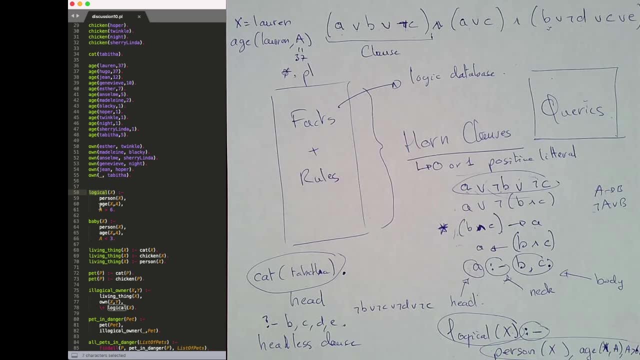 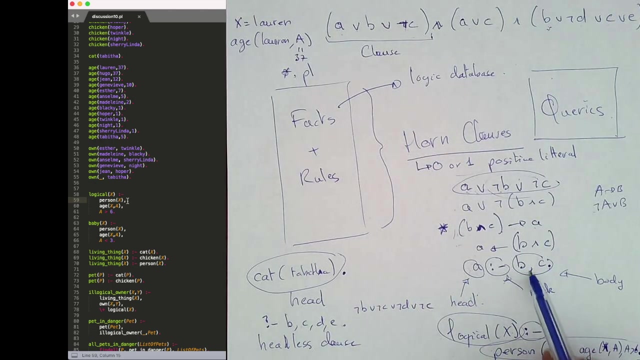 that's 37, uh, but it's. it is just a proposition that has to be true, right for this, the, the, the goal to be satisfied here. here, all the sub goals have to be satisfied because, again, each of these comma represents an end, right, remember, the comma on the right is equal to an end, logico, logically, right. so 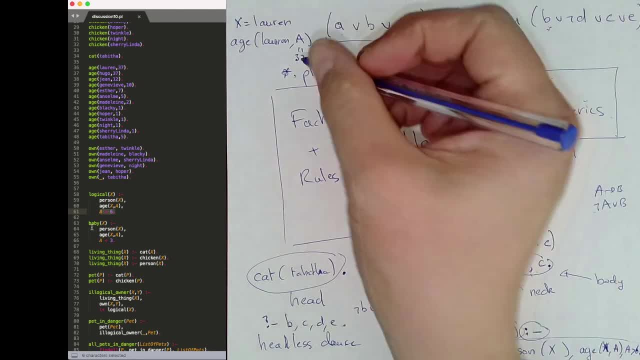 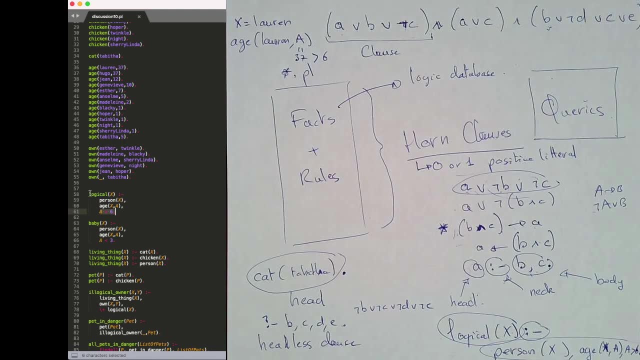 a greater than six has to be satisfied. it's the correct answer to the y and c equation, being able to satisfy the all of the sub goals. on the bottom linear case, right, 37 is greater than 6, so the third goal is satisfied, so the super. 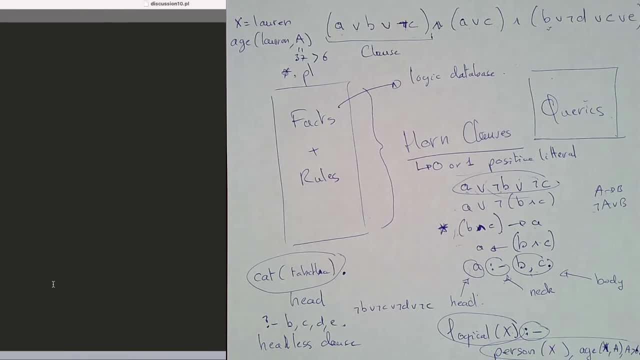 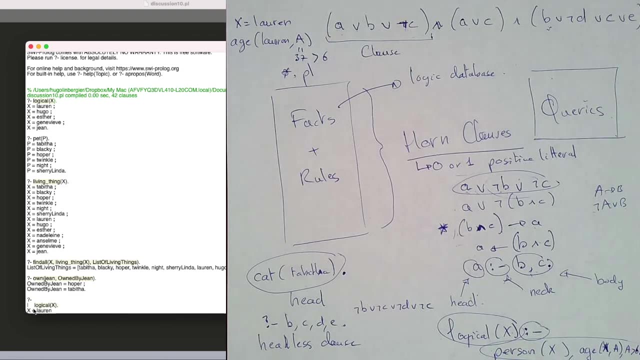 goal, if you want. the overall is now satisfied and so, because it is, and it was my goal- X is now unified. I mean, is now X equal lower and is offered as an option now, and this is an interesting thing, I don't know if you notice, but we 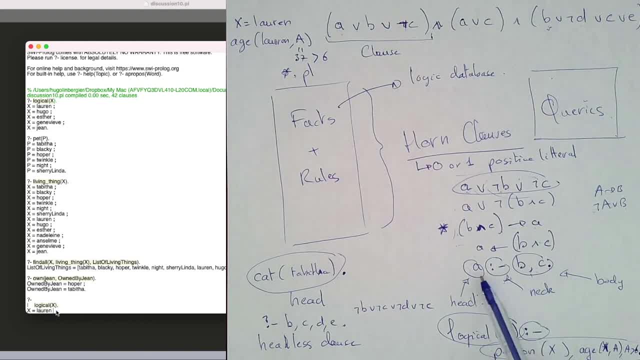 have no way to express, on the left side, the notion of or, because we have only, at most, one head. we don't have multiple heads. so I cannot say something like B and C, or a or D, and and I cannot add other options here. well, the way to all. 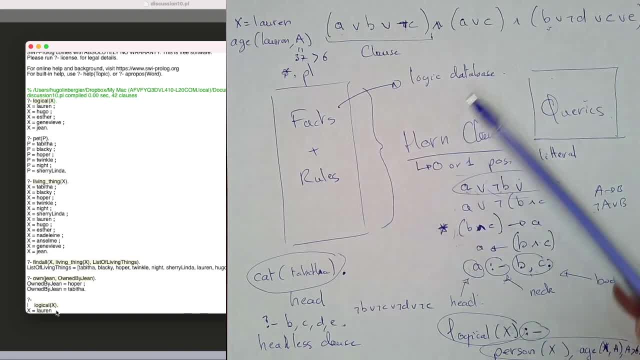 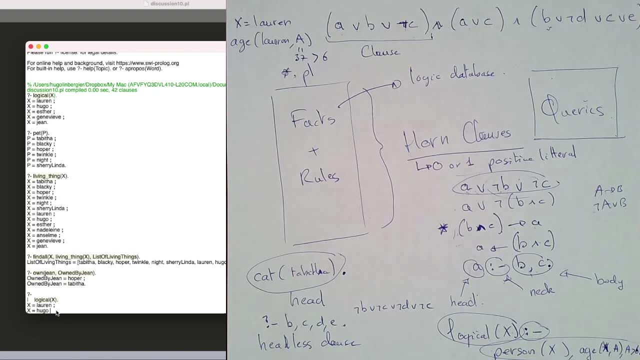 works and it's a bit tricky, but it really works within the calls through query. so here, if I hit the semicolon, which is equivalent to an or in the logic of prologue on the left, so in some sense, what, what I could write, is that the way we could? we could. 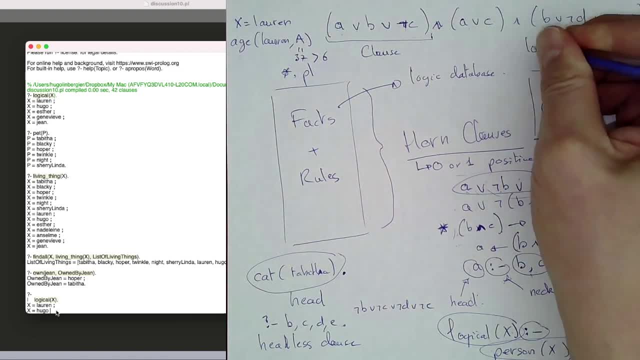 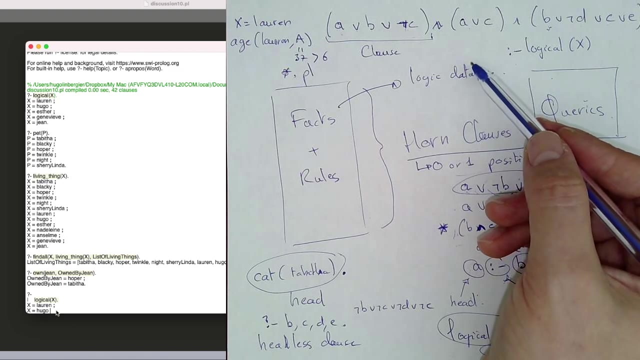 write this down. is that logical X is true? so that's again, that's hard, kind of like our headless question close here and and we, we, we put we can now in some sense we ask prologue to find the head to this headless close, right, so logical X is true if X equals. 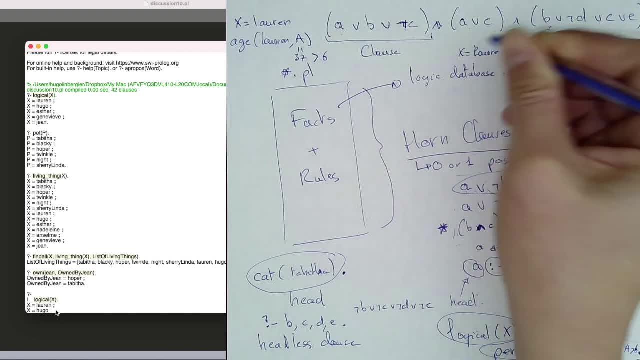 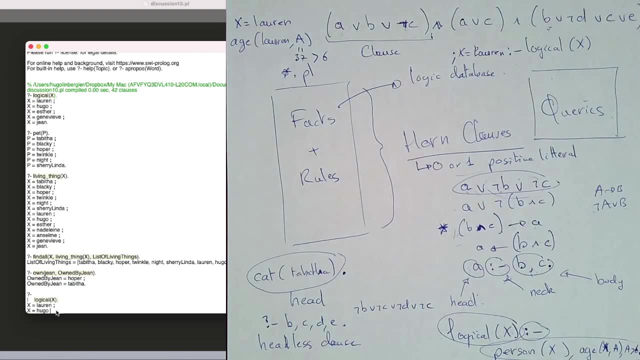 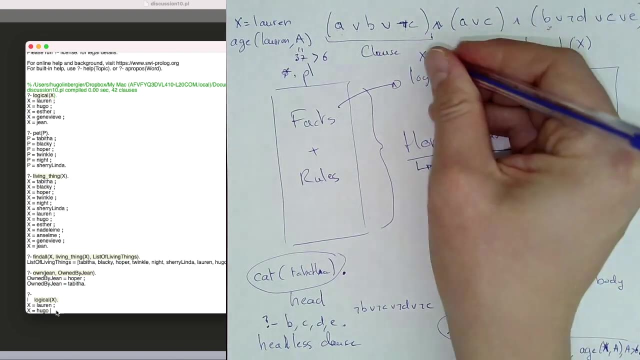 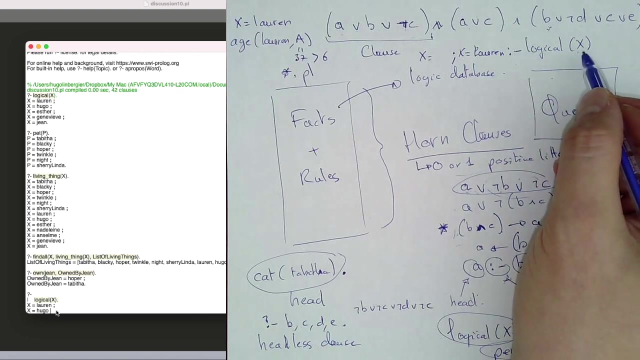 Lauren. but now we, we, the semicolon here that I'm putting on the terminal is- is basically asking: what find me another X such that this, this is, you know that, that such that logical X is true, so that you can think of the semicolon as an or and. now, 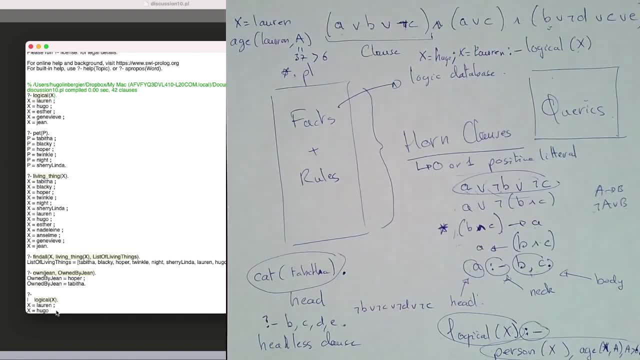 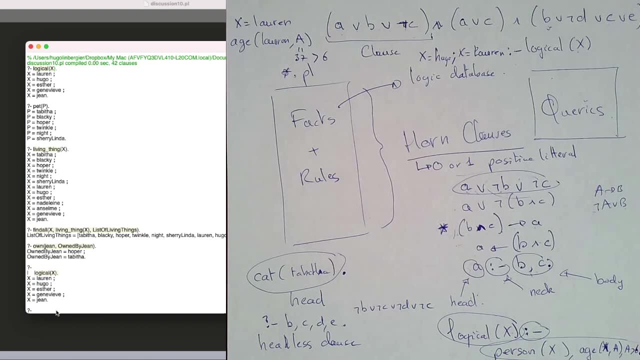 it. gave me another one. give me Hugo, and can we give me a bunch? right, but at some point is gonna, is gonna end up with a, with no more answer, and it's just gonna stop because it's it's it's over. some other prologue interpreters, instead of stopping, will tell you: no, there is no. 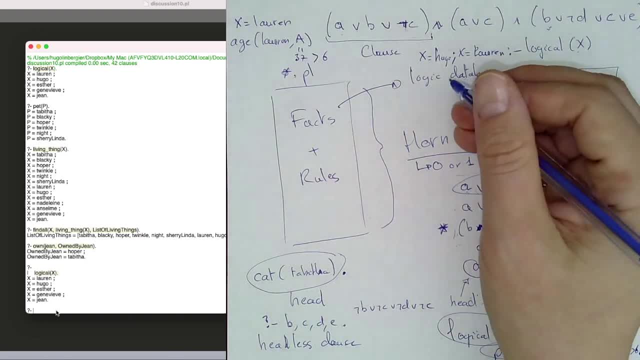 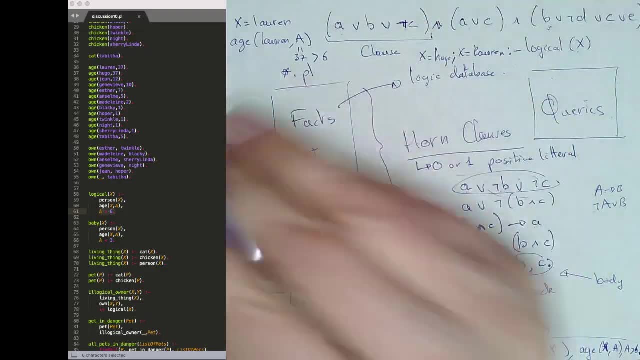 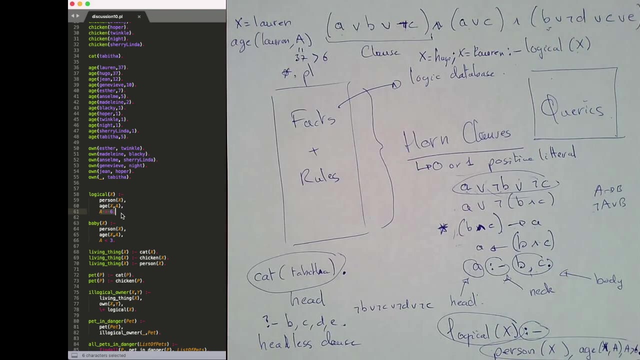 more answer. we give you an oen, sir, when you put the last semicolon. so anyway, what? what? don't worry too much about semicolon, that's kind of a something there's a bit a bit more complex to grasp, but what I really wanted you to to. 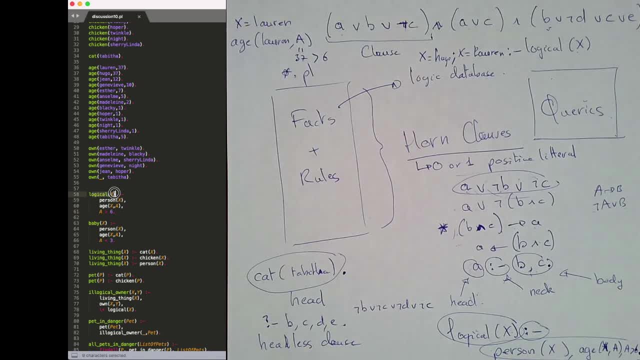 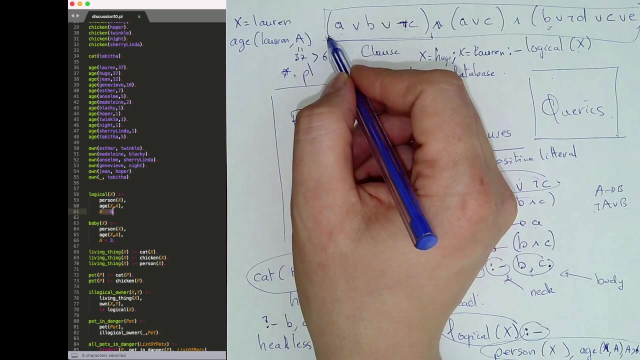 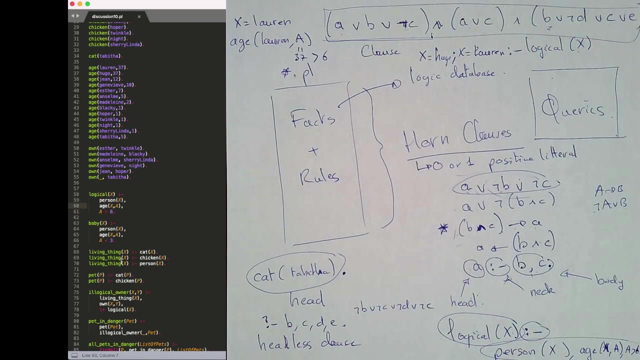 understood is how the resolution works and in some sense just have an idea of the linearity of it. I do not have to check every possible combination of truth values like I would do here. I do not have to check every possibility, I just have to take them one by one and you know if I have a query with. 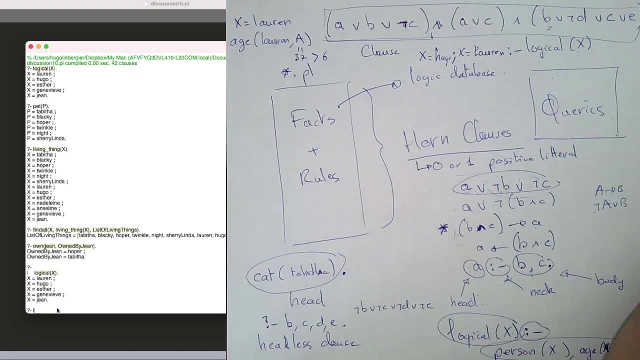 multiple propositions the way I have it here, right. it would be like this, for instance: here I want x to be logical and x to be also a pet. that's what it would mean, right? So now if I hit enter more in color, it tells me just false, Right? and the process in went through is the same. 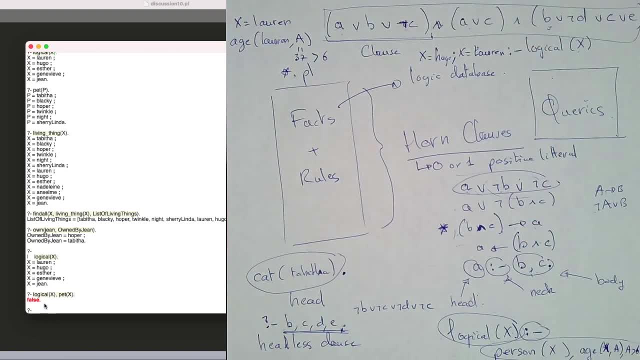 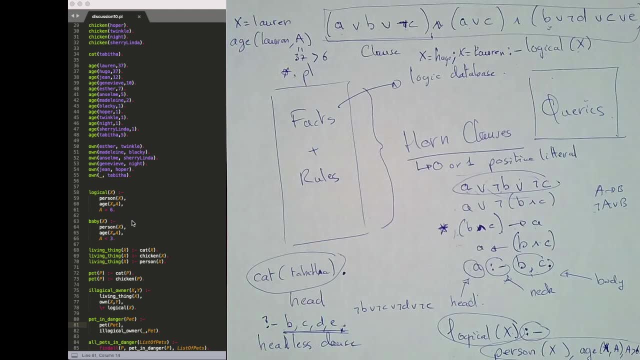 and the process through is exactly the same. It went through the process of: okay, I'm going to find a logical person, I'm going to go all the way down. it's going to find Lorinh first and it's going to try to unify Lorinh with the pet. 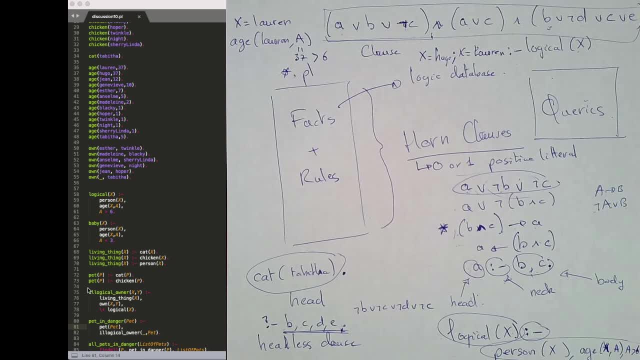 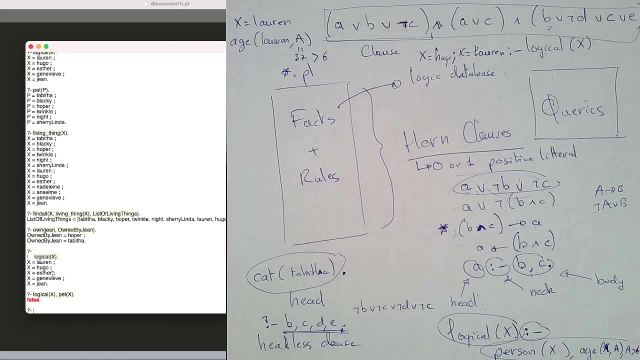 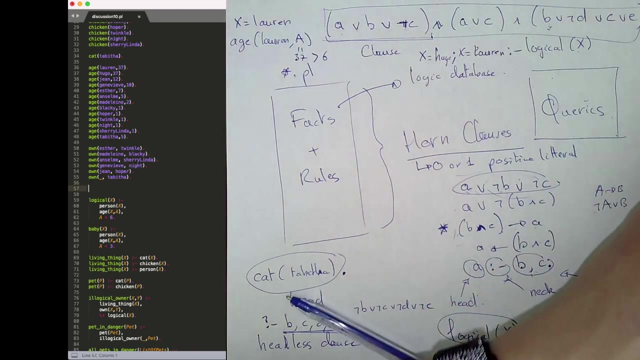 But the the problem is that the pets can only be satisfied. so it's going to try to look for pets right once, once. once it went through logical, it keeps going right because it has to satisfy both of this and actually doing this, or here putting a rule that is called logical pets. 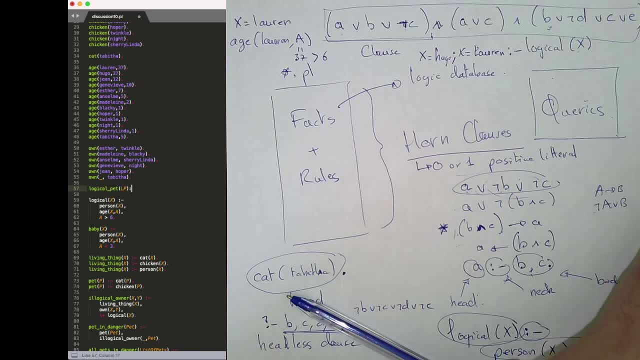 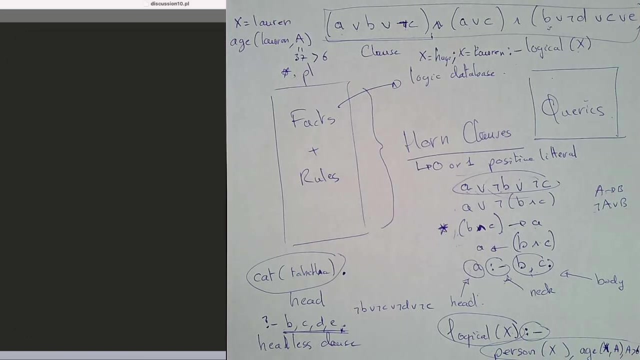 and saying: you know, logical LP and pet LP is exactly the same thing, right? if I write this rule in prolog and I then query logical pets here, it's the same thing as asking that here, right? because what I find is that the pet's are not the same as all the other pets. 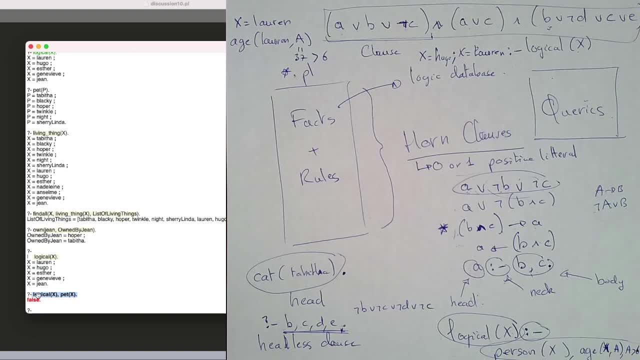 find here is in the body of my role here, right? so it's going to be the same process here. i'm going to try to unify, to find an x that satisfies that, that satisfies the goal, logical x, and it's going to return a bunch of of people and then for each of these i'm going to try to satisfy the goal. 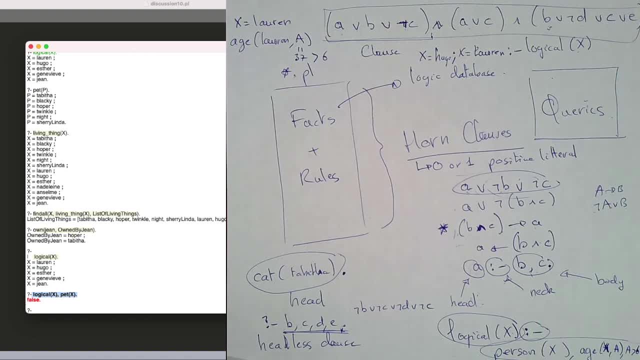 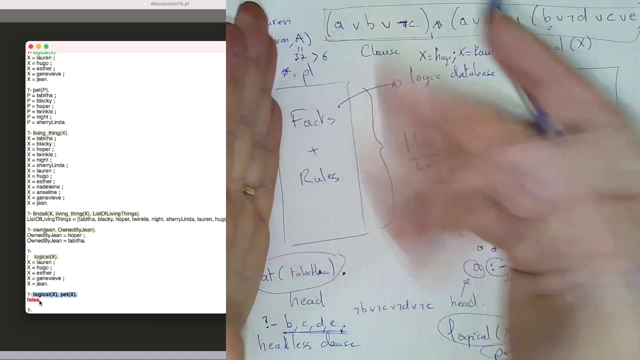 pet x, but none of them is going to work, so it just answers false. that means there is no uh satisfiable answer. okay, so that was my little overview. um, i i just really wanted you to get a sense of what is a prologue program really, to see it as a logic database with facts and rules. 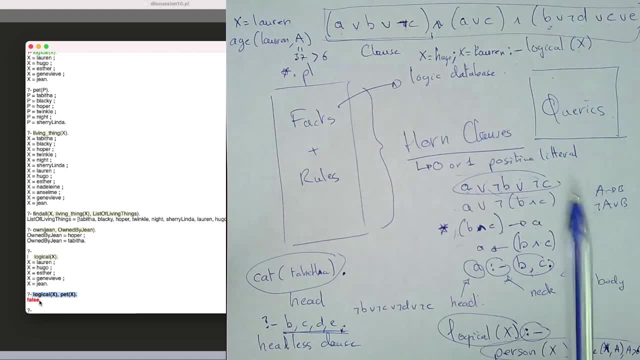 see how facts and rules have this thing in common, that they all have uh, one positive literal and uh and as many as you want of negative literal, and that the queries uh kind of complete in the set of home clauses, um, the facts and rules as home clauses, with zero positive literal. so headless, these headless. 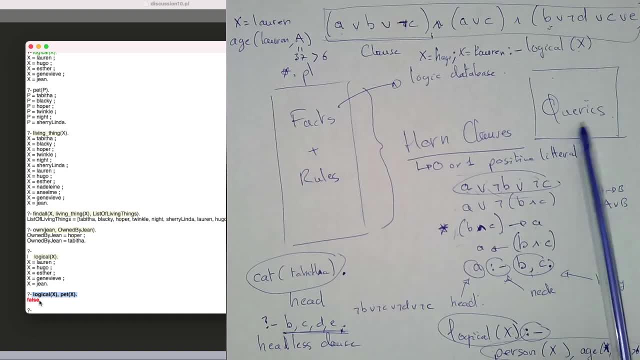 clauses, so they are of a different kind, and the way the way they are because they are like that we can take them really linearly, with taking each of these as one goal and we go through each of the goal to satisfy them in a linear way. this linearity is really what is foundational. it's what we call.